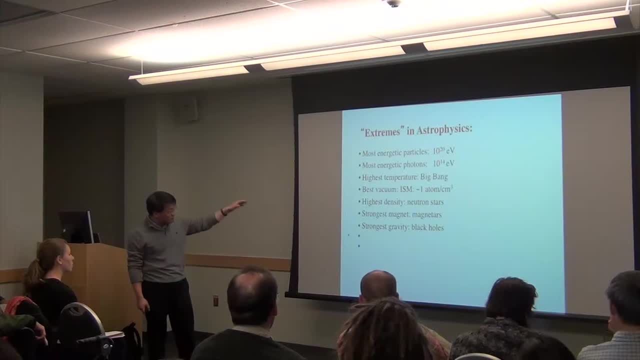 We study highest temperature in the universe, the best vacuum in the universe, the highest density, stronger magnetic fields, strongest gravity. We do all these fine extreme things. So today I'm going to focus on a particular class of compact objects. We call compact objects neutron stars. 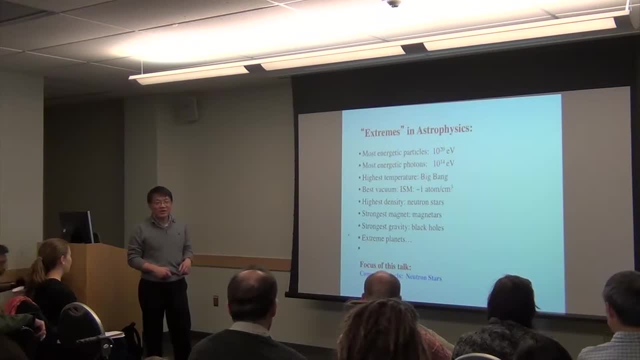 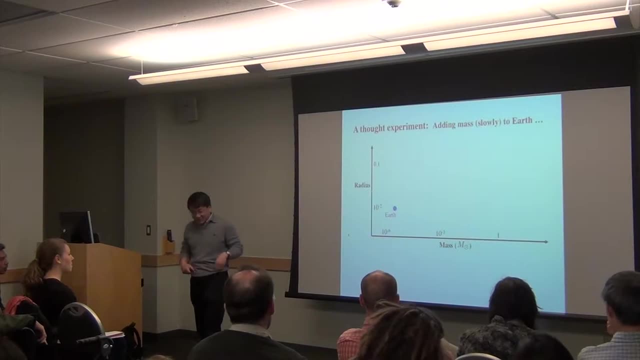 Okay, Okay, Okay, Okay. So to introduce you neutron star, let me, I like to. I'm going to walk you through a thought experiment. Okay, A thought experiment, Okay. So the way to introduction of neutron star. what neutron stars are? 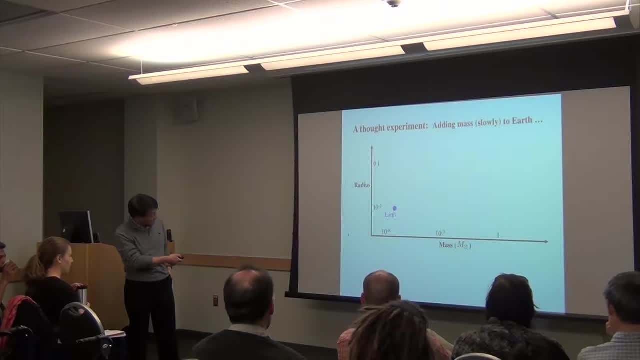 So here is a diagram: mass and radius: Right Right Earth is here, Right Radius: This is, I think, the solar radius. It's a unit of solar radius, Okay. Unit of solar radius, Okay. So Earth is a point here. 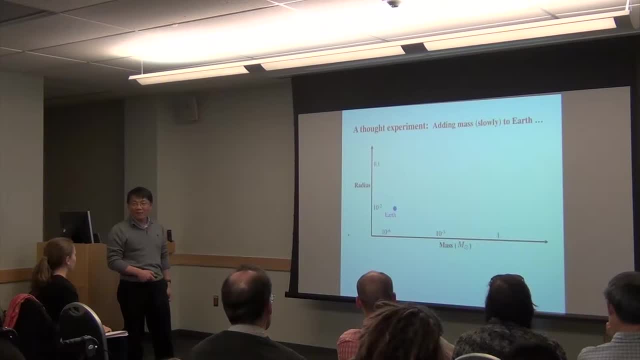 So now I'm gradually adding mass to Earth And I want you to go imagine how this curve, what's going to happen to this curve, Right? So of course, all you can answer: if you add mass to it, the mass increases. the radius will increase to the m, to the one-third power. 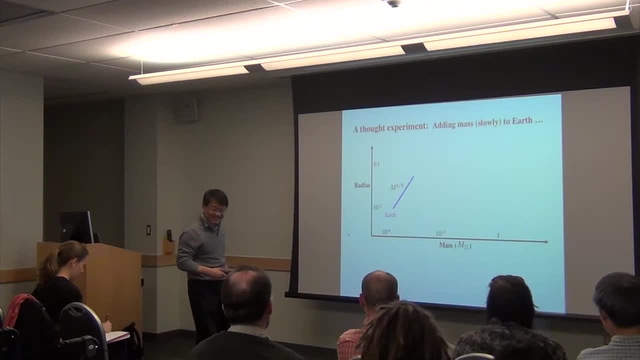 Okay, This you can derive. you should be able to derive it. Okay, The density: constant. Now, what may surprise you is that if you keep adding mass to it, at some point this curve will- Okay, This curve will turn over. It will not keep going on forever. At some point it will turn over Right around the mass of Jupiter. The reason for this is that if you keep adding more and more mass, the self-gravity becomes stronger. When you have more gravity, gravity wants to make things smaller. 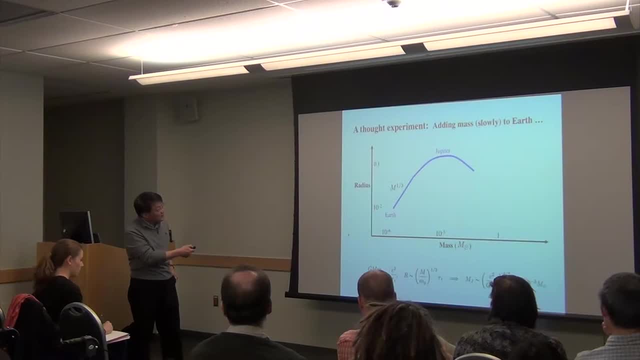 So when you reach the mass of Jupiter, the self-gravity is sufficient. If you add more mass, it actually becomes smaller. That actually may surprise you. Okay, Right, And I have some equations here I'm going to skip. If you're really busy, take them out. 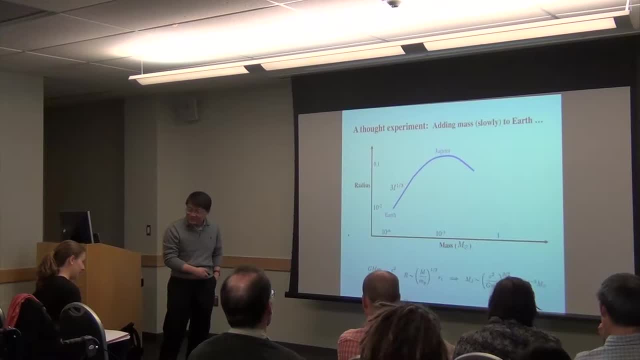 I can ask you later. I can ask you this: All this can be derived from simple physics, quantum mechanics, simple electromagnetism, Okay, Okay. So keep adding mass to it. At some point you reach the so-called Weydorf regime. 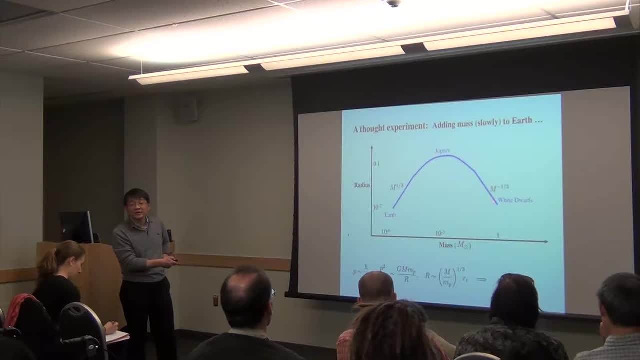 where you can actually derive a very clear relationship between the radius and mass, where the You add mass to it, the radius decreases as m to the minus one-third power. So in this case, Weydorf you have. It's basically you can see here Weydorf has mass about solar mass, mass of the sun. 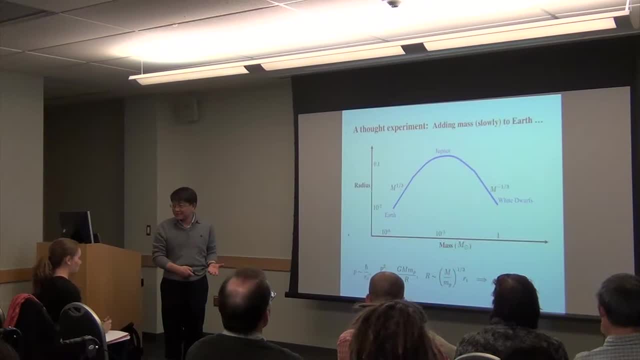 but radius, roughly about the radius of Earth. So it's very compact, Very compact. So Weydorf is the first kind of compact object we see in astrophysics. It's very compact. So what's happening here? yes, there's a lot of gravity, a lot of mass packed in a very small range. 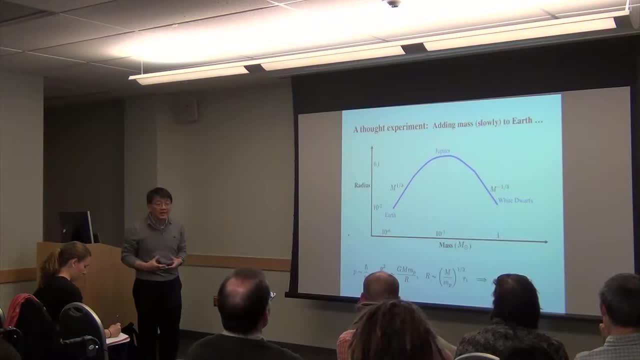 so the self-gravity is very strong, right? So what's supporting it against gravity In this case? in the case of Weydorf? what's supporting this Weydorf, against gravity? It is quantum mechanical pressure, Zero point energy, so-called degeneracy pressure, right? 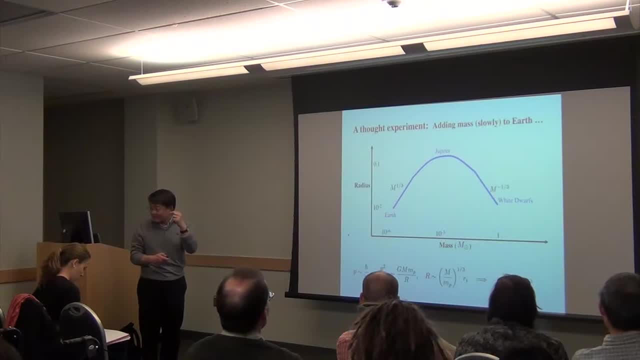 The electrons keep moving, even at very low temperatures moving, And that moving manifests as the pressure that's supporting it against gravity. So the quantum mechanics degeneracy pressure it's supporting Weydorf against gravity. Okay, And if you keep adding mass to it, at some point it's curved. 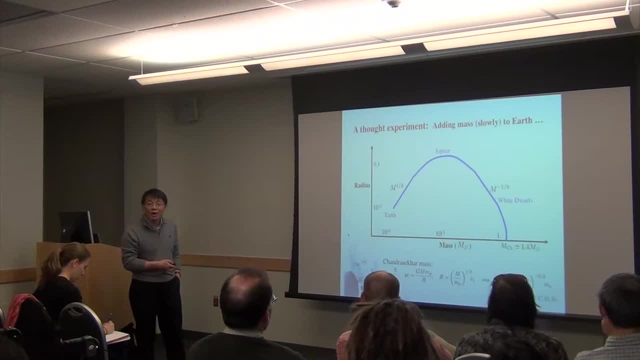 It turns over to a limiting value, and that value is one of the two most important numbers in astrophysics, The first one being the- you know double-cost how fast the universe is- And it is, I claim, the second most important number in astrophysics: the Chalasikon mass limit. 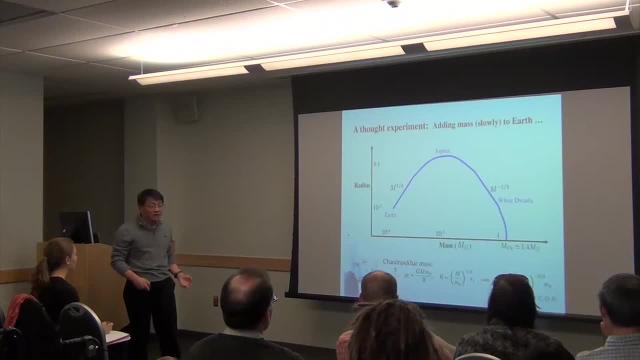 So, namely, at some point, this mass has reached its limit. You cannot go beyond that right. The reason for this is that, as I said, white water has a lot of gravity. It's being supported against gravity by this zero-point motion. 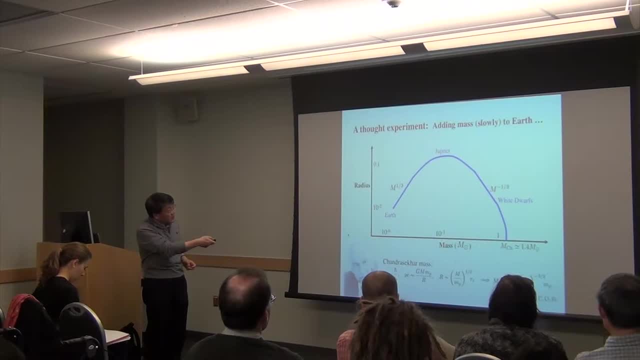 Right, Right. So if you have a lot of gravity, if you keep adding mass, it becomes more and more compact. You have more gravity, But so you have to speed up the electrons to make it to support it. But of course we have no special relativity. 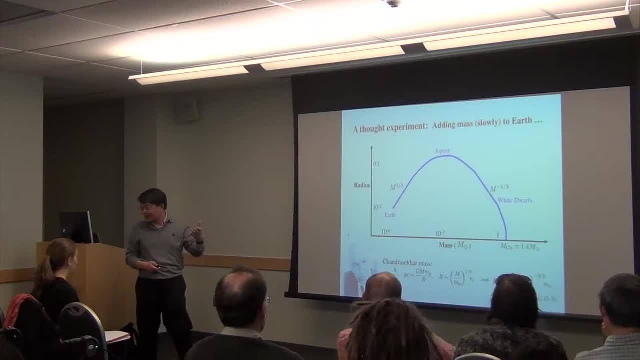 There's finite speed, the upper limit of speed, the velocity of particles. So therefore, at some point, when you have so much mass in a small region, your electron can only move that far, that fast, Right. So that's the reason. 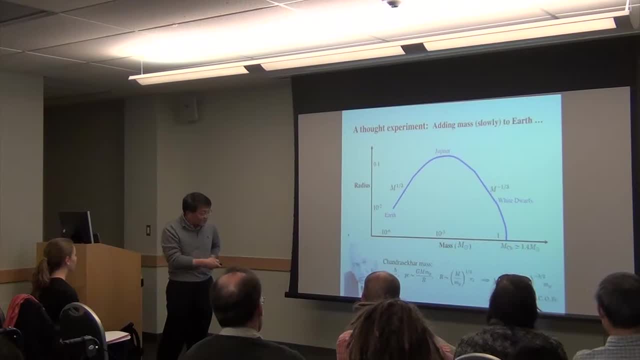 That's the reason for you to have this maximum limit, mass limit. So this is limiting mass. okay, in Chalasikon, So you can see this. actually this number, the 1.4-tholomaths, actually can be expressed. 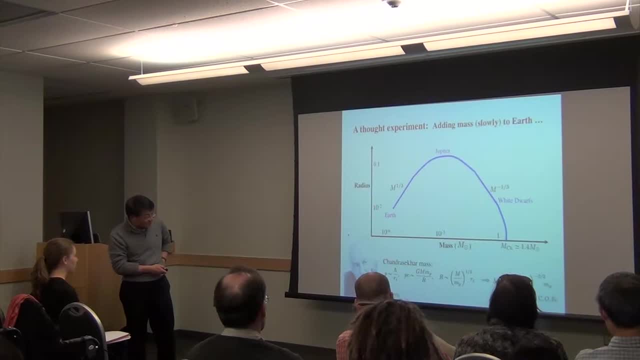 in terms of fundamental constant, Because this is the main fundamental constant. You can see, it involves g, gravity, photon mass, c, special relativity, h-bar, quantum mechanics, Right, So this is a beautiful marriage of all these three things, okay. 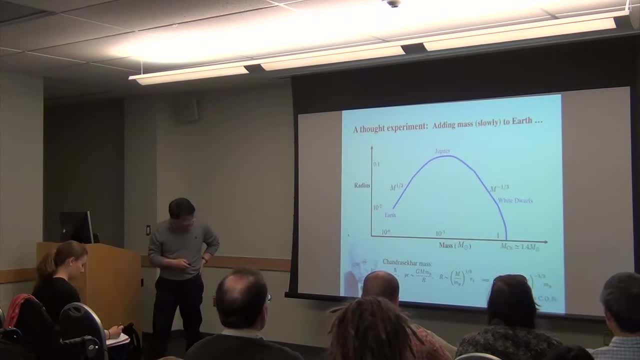 and giving rise to the Chalasikon mass limit. Okay, So now let's continue the experiment. If you keep adding mass to it, dripping mass to it, you've reached Chalasikon mass limit. What's going to happen? 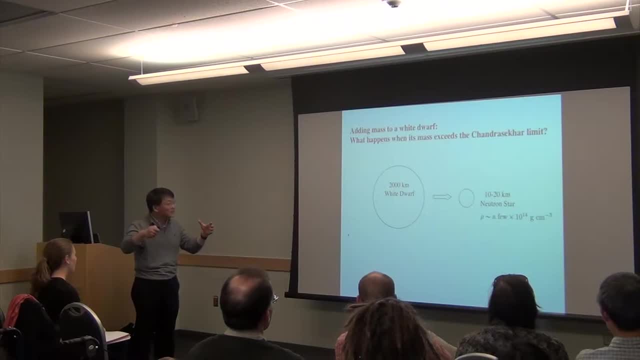 Well, it can no longer hold it together. It will collapse Because what this is going to do, it can no longer be supported against gravity by this quantum mechanical motion electrons. It has to collapse. Okay, It's going to collapse. It will collapse all the way until the neutron photon in the matter. 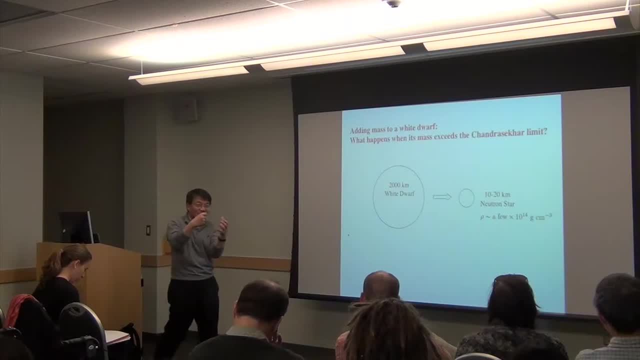 it's going to collapse. This is saturation, So this is so, so it's going to collapse as a result of this elevation. There is this that I Amanda scenario gives a important point is time in centimeters, This current, this constant. 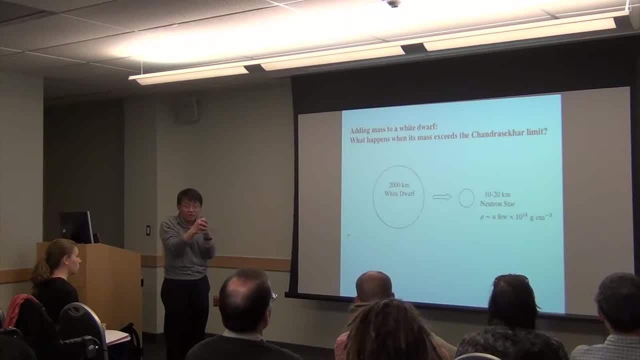 Okay, so all the neutron protons are squeezed against each other. they are very tough. Okay, so in the case of neutron star, you have even more, even stronger gravity, but it's supported against gravity by this nuclear force, force. Neutron protons touch each other, Alright. if you keep adding mass to it, well, you get different possibilities. It's a bit uncertain because we don't really know what's happening when you squeeze neutron protons together, how they interact with each other. There are some uncertainties In nuclear physics. you are in the regime where you are squeezing neutron protons together, so there are some uncertainties, right? So, depending on the detail of the physics of how neutron protons interact with each other, when you squeeze them, you get different behavior. 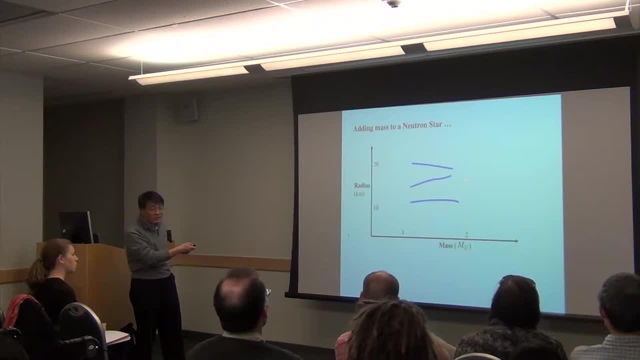 So if you add mass to it, sometimes it increases, sometimes it decreases, depending on the micro-physics, nuclear physics. Okay, right, So we are probing this regime where you have very dense matter, nuclear matter, bulk dense matter, squeezing them in case of neutron star. Keep adding mass to it, regardless of the detail of nuclear physics. all these curves will turn over, reaching a limiting value, right? The actual value of this maximum limits depending on the nuclear physics right. So some nuclear physics will give you maximum mass. what? 2 solar mass? some may give you 2.5 solar mass, right. 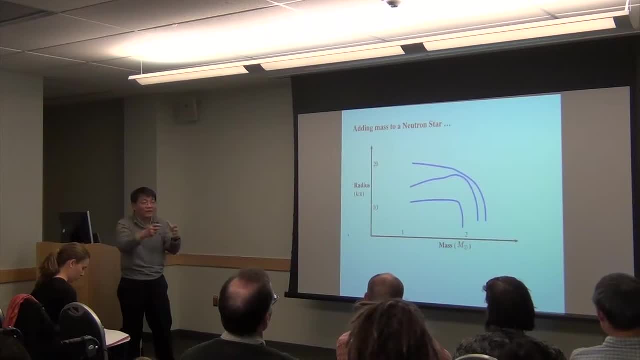 So what I'm saying here? if you add so much mass to it- because neutron are so compact, so gravity is so strong, even nuclear forces cannot support it- Add so much mass to it. okay, So this is my cartoon, but people actually calculate this kind of thing. Professional nuclear physicists actually calculate this kind of thing. You can see. here is the actual mass radius diagram. I mean it's inverted from my version, but it's very similar. It's the same thing. You can see, all these different complicated curves represent different assumptions about how neutron and protons interact with each other, right? So there are a wide range of theoretical models how neutron and protons interact with each other, right? So that will give you a different prediction of how the mass and radius depend on each other, right? But regardless of how uncertainty in nuclear physics all these curves have a maximum value. You can see right. This particular model predicts the maximum mass of neutron star is 1.4 solar mass. You cannot have more. but if you use different nuclear physics models you will get maximum mass of about 2.2, right. 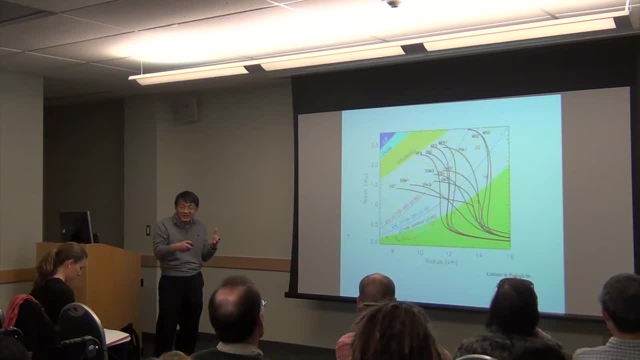 So you can see, this is where, if you actually observe, be able to measure the mass and radius of neutron star, you can in principle constrain the nuclear physics of nuclear matter. It's strongly impacting nuclear matter, right, And in fact people are doing that. 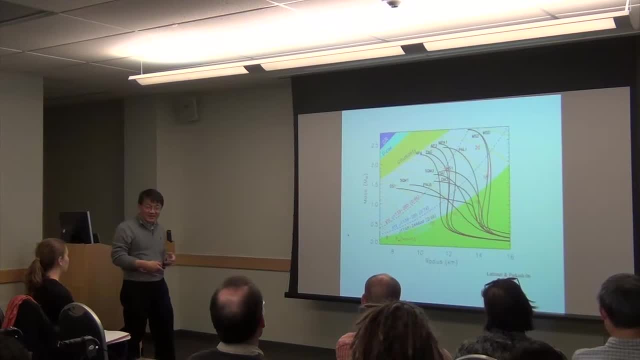 Astrophysicists have been doing this for about 10, 20 years or so. They will continue to do so in the coming decades. It's a new experiment. I'm going. I'm not going to talk about it. People are trying to do this kind of thing. 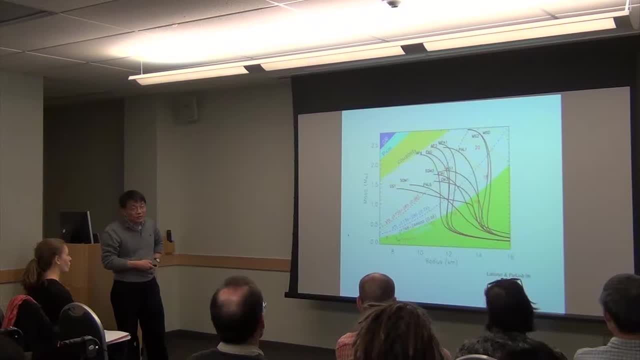 Okay, So let's continue. Well, you can actually, given that there's maximum mass for neutron star. so if you keep adding mass to it, you can ask what's going to happen. What's going to happen to that mass? Well, it's going to collapse. If the mass exceeds its maximum mass, it will collapse. Even nuclear force cannot support it. This thing will collapse all the way to black hole. And black hole is the third kind of what we call compact object that we encounter in astrophysics. 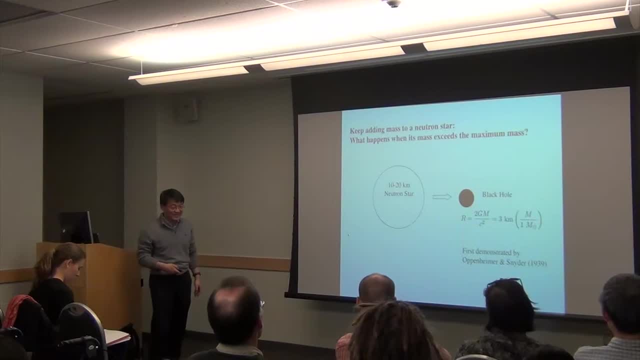 Okay, Now I'm not going to talk about black holes in this lecture, So let's see. So the inventory: when astronomers talk about compact objects, we're talking about white dwarf, neutron star black holes. They are very compact, right? 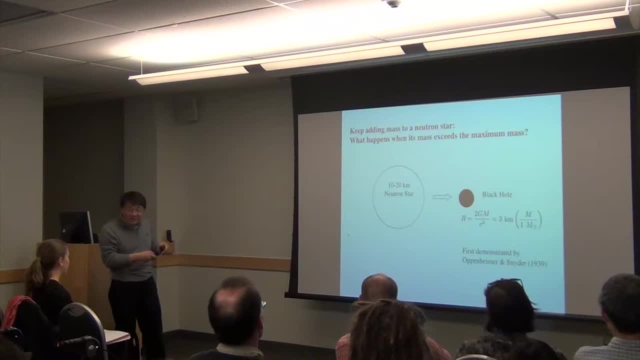 To various degrees. Okay, So that's my thought experiment. Okay, So, starting with a rock, gradually adding mass to it, you get white dwarf, neutron star black hole And, of course, in reality, in real astrophysical universe, this is not how you form neutron star black hole, right? 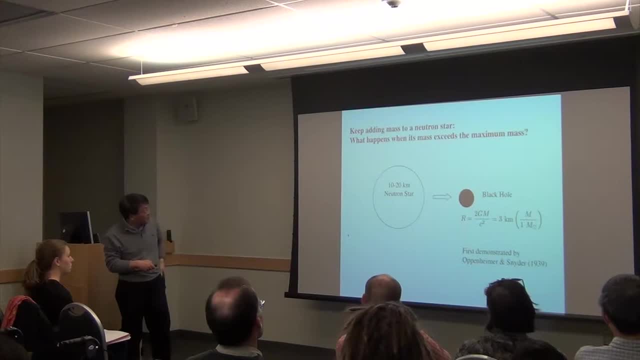 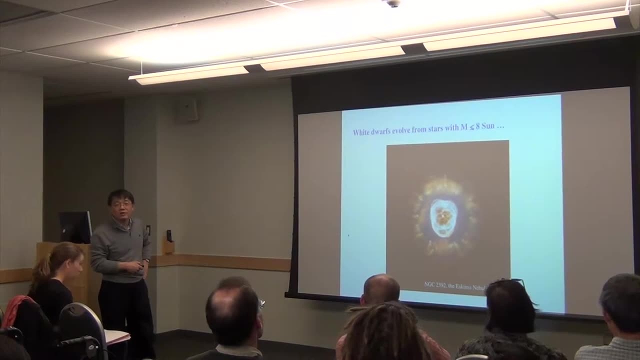 So I need to tell you a little bit how you form neutron star black hole. Just quickly. Just make sure it's a complete picture, right? So what we think is that white dwarf is a result of stellar evolution. All these compact objects are the remnant of stellar evolution. 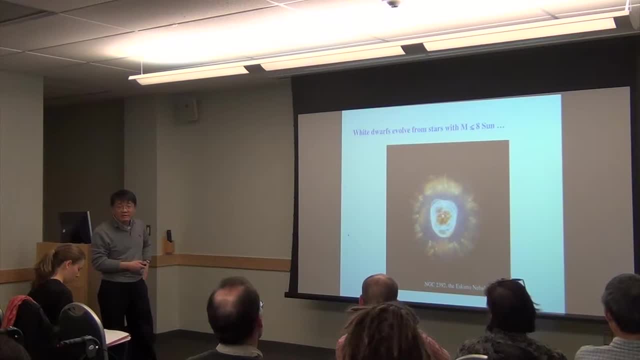 So if you have a star with mass less than eight solar mass, our sun, our own sun, right, It's one solar mass. Eventually, after it runs out of the nuclear fuel, the central portion of the sun will eventually collapse to become white dwarf. So our sun, that's, the fate of our own sun after some billion years? Okay, No need to worry. Eventually, this portion of the sun will become white dwarf, Okay. And neutron star. it's a remnant of a more massive star. Namely, if you have a star with mass greater than eight solar mass- 20 solar mass, for example, this massive star, eventually the central portion of the massive star, will eventually become a neutron star, collapse to form a neutron star. 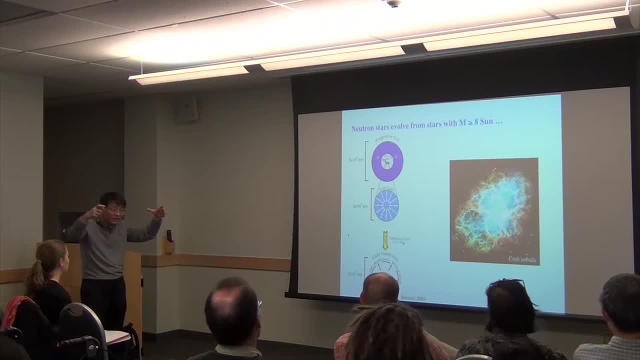 Okay, It's doing this in a spectacular way. Before it dies, it becomes a neutron star, It explodes, The whole star explodes, making a supernova, And this, of course, is another completely different topic. I don't want to go into it. 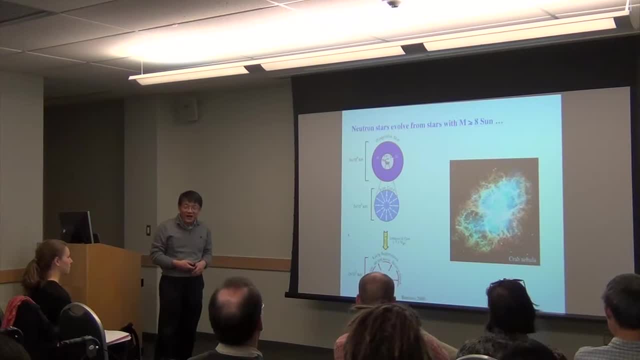 Right. So massive star dies in a spectacular way by giving out explosion and showing off itself, and then the central portion becomes a neutron star And black hole. we think they form from even more massive stars The central portion, the more massive they become black hole. 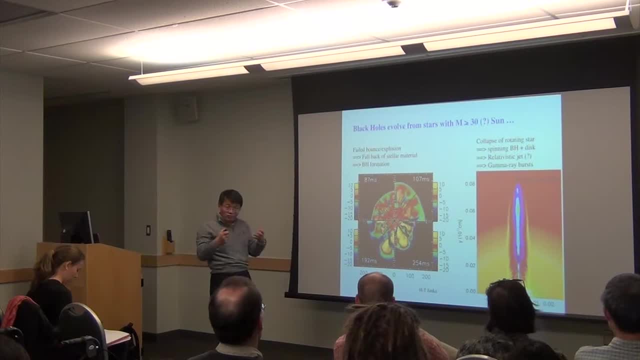 Okay, So in astronomical, astrophysical universe, these compact objects are the remnant of the evolution of normal stars. Okay, Okay, neutron star is one particular kind of this. Okay, So this is a complicated slide that I don't want to go into. 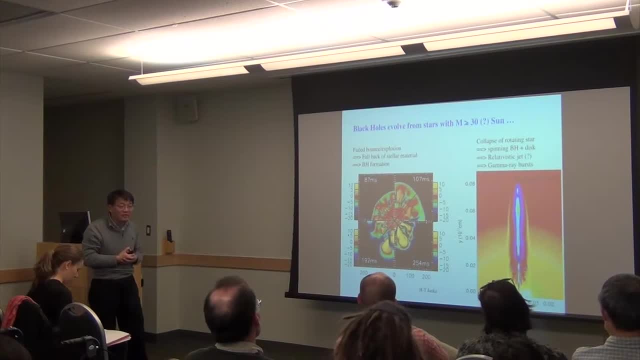 When you form a black hole in this massive thing, collapse, you know, you can give rise to all kinds of phenomena that we observe. I'm not just making this up, People. actually there are observational, you know, evidence of this kind of thing. 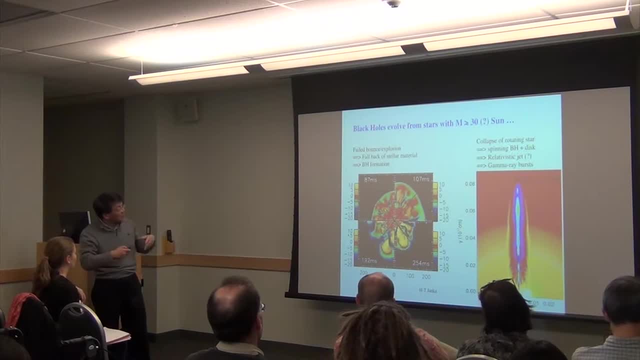 For example, they may. when you form a black hole in this particular way, you may produce so-called gamma-ray bursts. Bursts of gamma-ray you can observe. These have been observed. Okay, So that's my sort of my introduction of what are these compact objects? 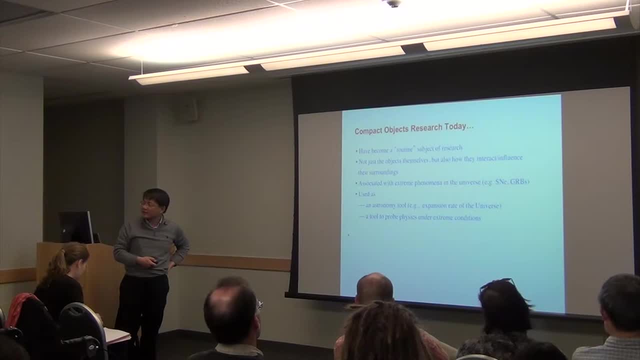 Right. So it's really. if you think about it, these are really exotic objects. You pack solar mass, solar big mass, into a very small region, Right? In the case of neutron star, one solar mass, pack them into 20 kilometer radius. 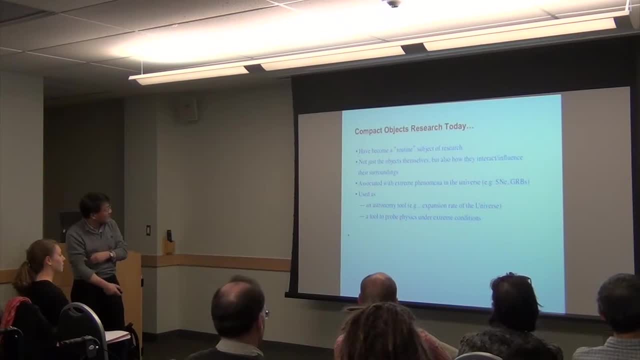 which is very, very dense. So it's a very exotic object, But these days these have become a routine subject of research. It's showing the progress. We have been studying this kind of object for the last so decades now. 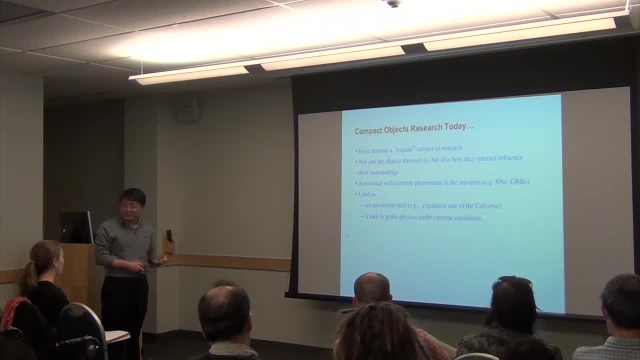 The evidence. these are not fictions. We have observed various manifestations of these compact objects in various ways, Right And we. when we study these compact objects, we are not only interested in these objects themselves. So we've done black hole by itself. 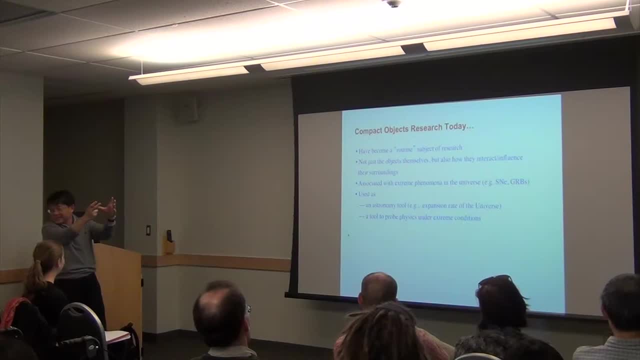 Black hole by itself it's very difficult to study. It's dark Right, It's pretty dark Right We. but the interesting thing is They can manifest themselves when they interact with the environment. So we are only. we are also interested how these, for example, neutron star black hole. 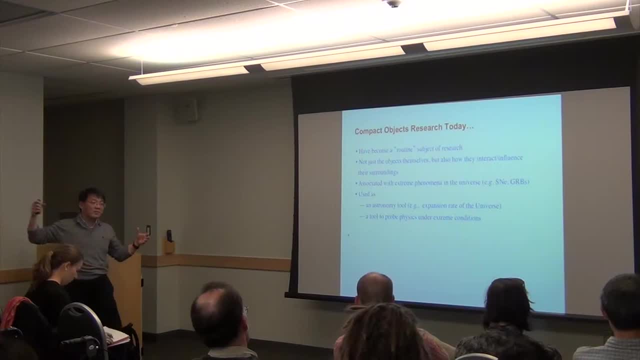 interact and influence the surroundings. So when you, for example, in the case of black hole or neutron star, if you dump mass into it, they can shine in bright x-rays. They can, they can make explosions And give you a lot, give you emit x-rays, for example. 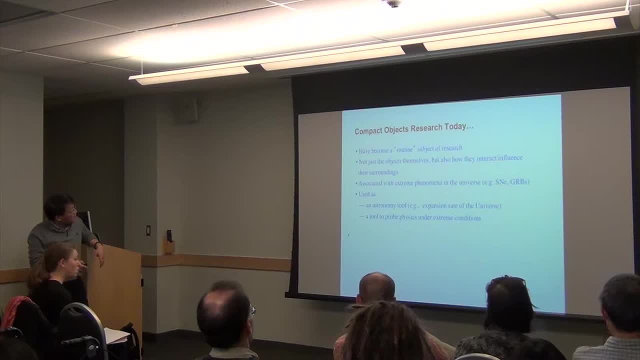 Right. So we study those things And these compact objects are now associated with black hole. These are now associated with many extreme phenomena in the universe Right, Such as supernova explosions, where the neutron star forms The masses, but masses are dark. 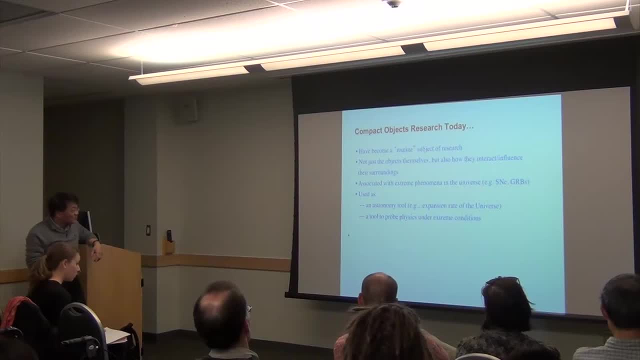 It's the evil of the explosion- And gamma- it was only briefly just mentioned by me- Right And and increasingly, these compact objects have been used as a tool to study the universe, Study astronomy, For example. some of you might have heard about, you know, universe, universe expanding. 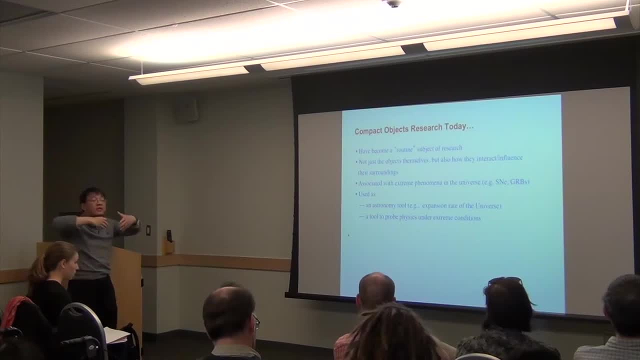 It's, it's bending in the accelerated way, the expansion rate is accelerating, And that's how do we know that It's actually used some of these compact objects, the, the standard candle. So so, the supernova white dwarf, the quaking white dwarf, the standard candle. 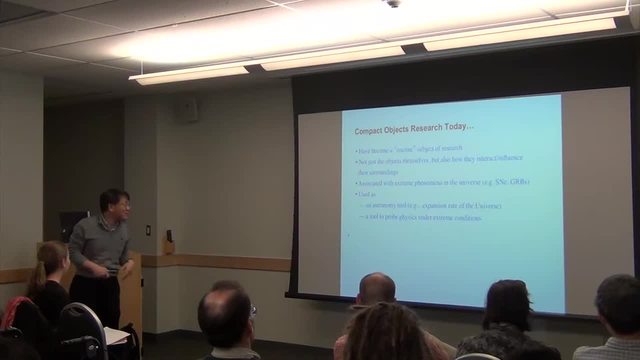 So, using this compact object, one can probe the whole universe And, in addition, these compact objects have been used as a probe to study extreme physics, Physics under extreme conditions, And it's not so surprising, because I I mentioned this. These are very extreme objects. 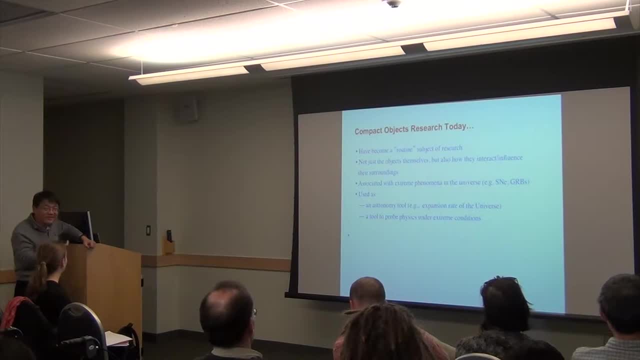 Very dense, Very a lot of gravity, A lot of very high density And a lot of magnetic field, Right? So? so this is the scene I want to focus on today In the remainder of 45 minutes. Okay, 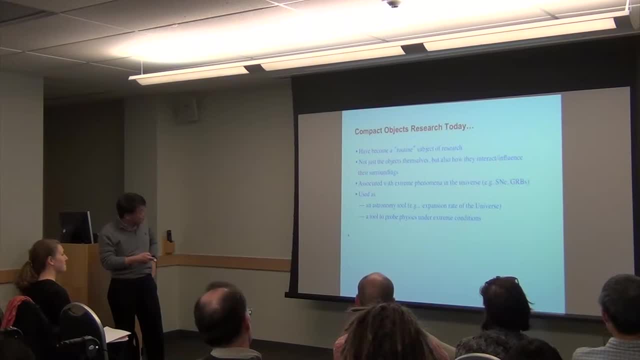 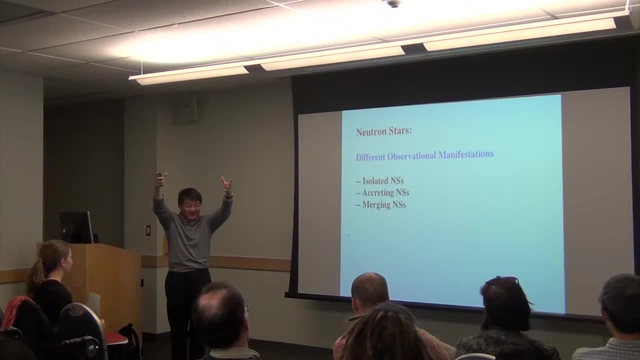 So now for now, for now, I'm going to focus on neutron star. now, Okay, So neutron star, So one solar mass, 10 kilometers. Very boring, just sitting there in space. How do we observe it, Right? How do we manifest themself? observational? 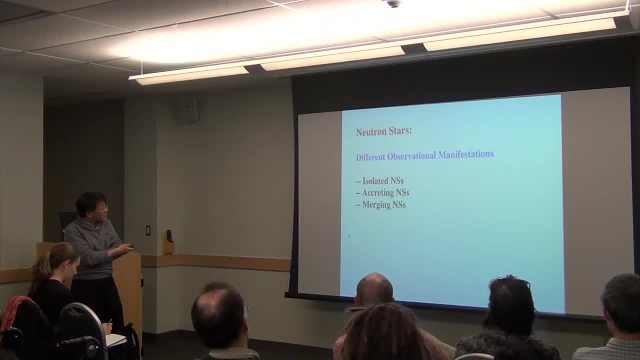 There are many different ways they can manifest in many different ways There are, so there are several different types. So, roughly speaking, you can have isolated neutron star by itself in the Earth. You can observe them. You can have the quaking neutron stars. 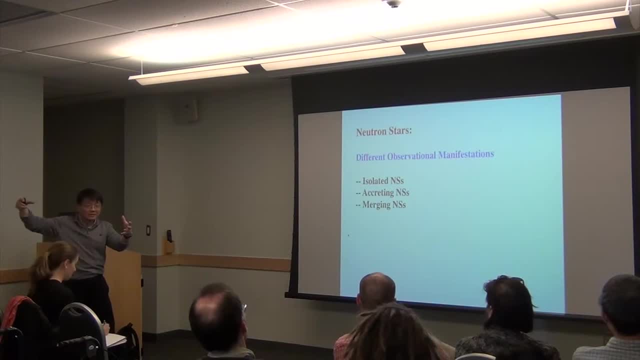 You have basic neutron star. they are in the binary system, The quaking mass, Sucking mass of the binary companion, So making bright X-rays. You can have two neutron star coming together, Merging, Generating interesting things. So I'm going to talk about each of these things in turn, okay. 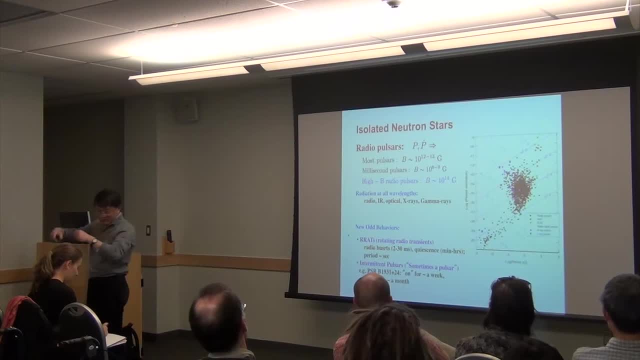 So let's first talk about isolated neutron star. Neutron star in isolation. So these have been studied over the last 40 years or so. So the most prominent way these isolated neutron star can manifest themselves is through radiopulsar. So radiopulsar is a particular kind of neutron star. 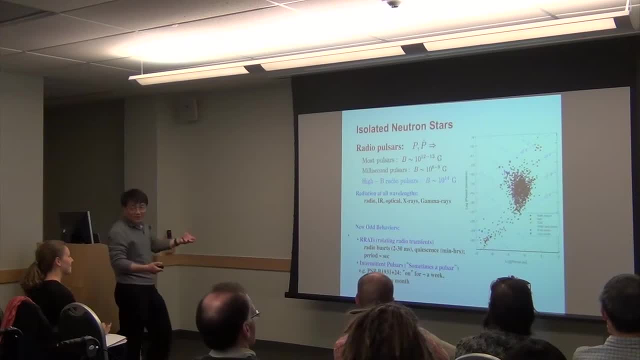 That's one particular way they manifest themselves, So radiopulsar, of course. Joanna Rankine is an NGA expert here. If you want more detail, you can ask them. These are basically. you observe them, they just pulse. 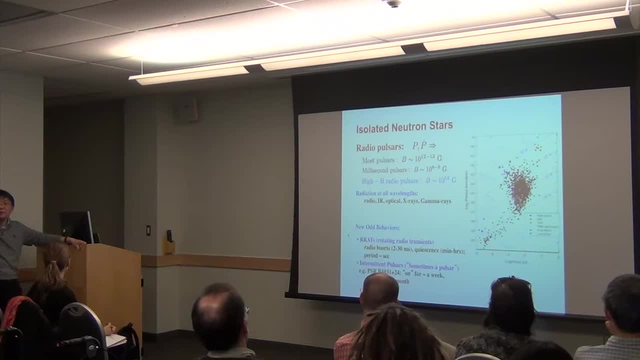 You know radiopulse coming out in a regular pattern, basically You know every two seconds they pulse. So by now they are now almost close to 3,000 pulsars have been detected. Many pulsars have been detected. 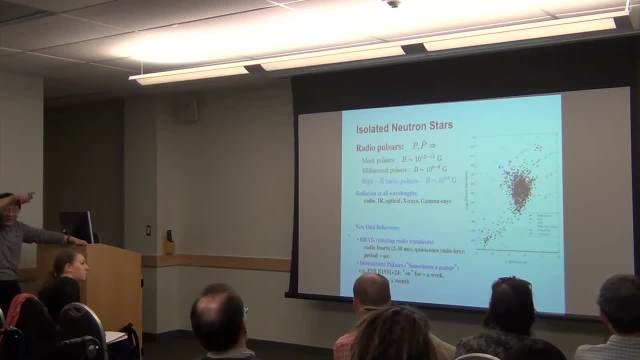 And When you observe radiopulsars, these regular pulsars, right, Two things you can detect very quickly, relatively quickly. The first thing is the period. You observe the period, You know how regular this pattern is right. 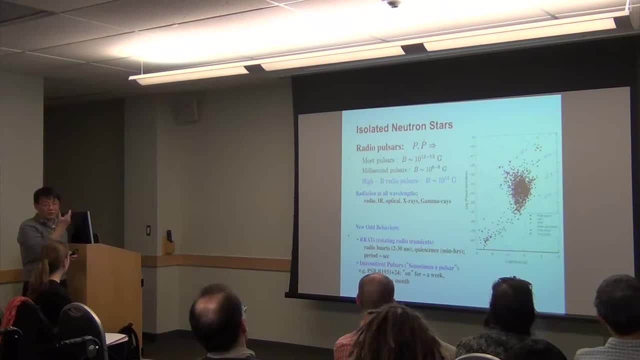 So this period, we think it has to do with the rotation period of the neutron star: Right, Right Rotation period. Basically, what happens, roughly speaking, is: you have a light bulb, you have emission, beam, emission coming from the star. 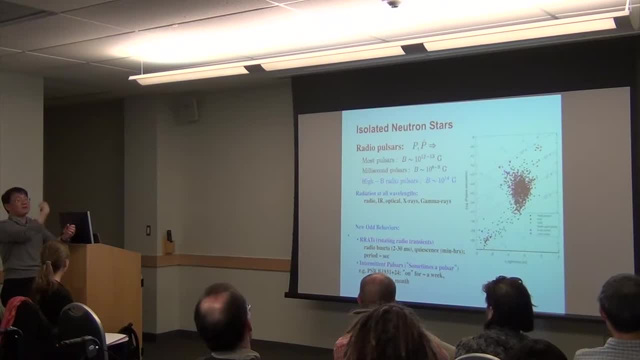 So you observe what happens to be at the line of sight. So every time the light bulb is coming towards you, you see the pulse Right. So the observed period of the pulse is the rotation period. That's one thing you can get very quickly. Another thing you can also get relatively quickly is: you monitor the pulsar for some time, You can immediately see how you can see that the period is not constant. It's actually changing in time. So you can measure the p dot, the period, the relative. 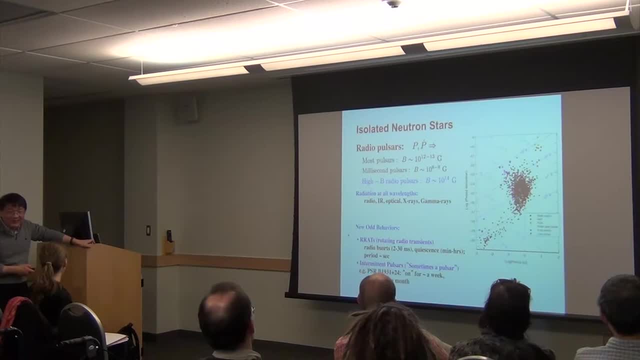 How fast the period is changing. P and p dot. Okay Now, just from these two numbers you can get a lot of things. The most important thing from this number is the magnet field of the pulsar, The dipole magnet field of the pulsar. 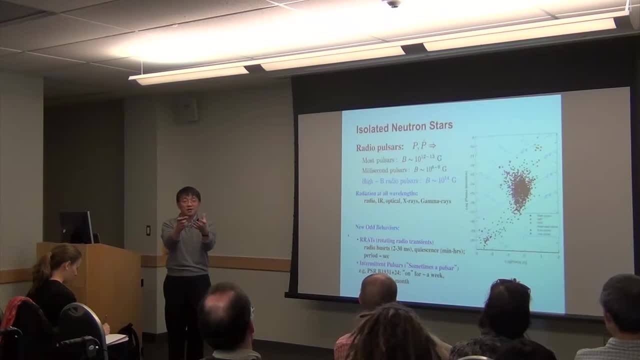 How do you do this? The concept is following: Right, You have a star which is rotating. Right, The star has a magnet field. So, roughly speaking, you can imagine that it's a magnet. It's a magnet, You have a rotating magnet. 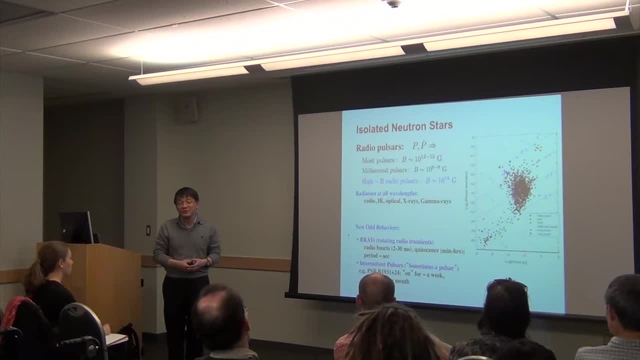 Well, the combination of rotation and the magnet field give you magnetic dipole radiation Right. So you assume this spin down, the p? dot, is due to radiation of of magnetic dipole radiation. Then you can. you can immediately infer how strong the magnet is. 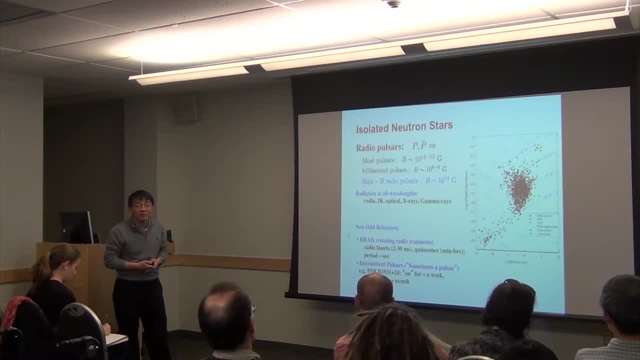 Right, What the big, what the field, dipole, magnet field of, of pulsar is, Assuming that you know the mass of neutron star, you know the radius of neutron star, You, you, we don't really know, of course. 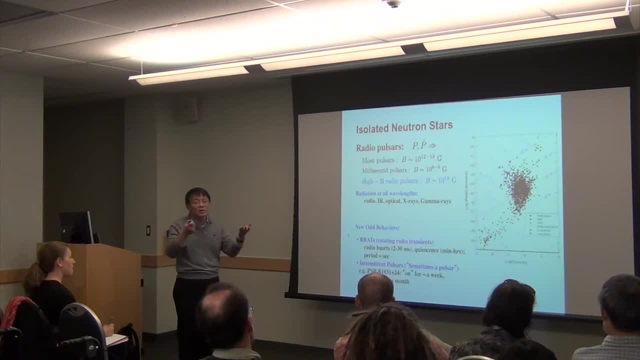 We don't know the mass, We don't know the radius, But we have rough idea. It's about, about solar mass. It's about ten kilometer radius. So more or less there In order of magnitude, Right? So so by measuring these two numbers, p, p, dot- you can immediately infer the dipole. magnetic field of neutron star. I should really emphasize this is a really dipole field. Okay, And so what you find is that most pulsars, most pulsars, have a B field in this range 10 to the 12 to 10 to the 13 dots. 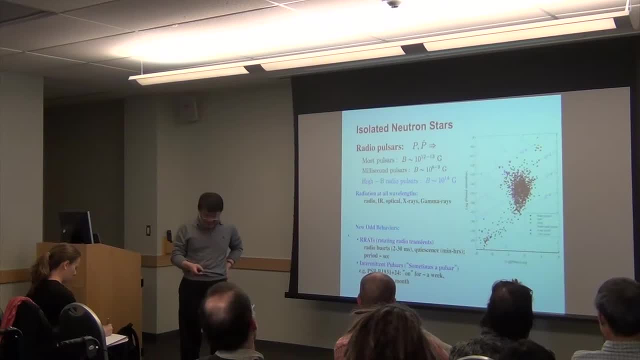 Now how big this is. Do you have an idea how big this is? The magnet field that earth on earth's surface that drive your compass is about one gauss. Okay, One gauss. This is a little tall, And if you put your magnet on your refrigerator door, that that that kind of magnet it's. 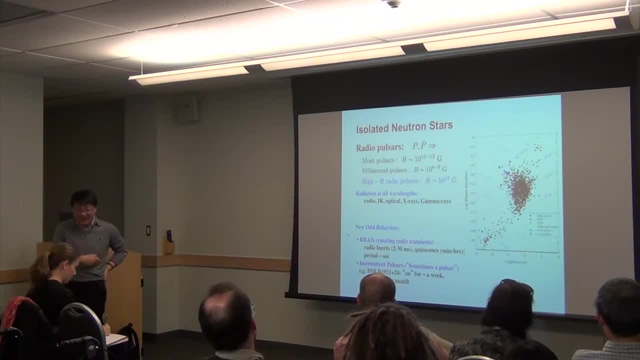 about 100 gauss. Okay, So this is many other magnet larger than that. Okay, To tell you how extreme we are, de extreme magnet field we're dealing with. Okay, So these are. most of the pulsars have this kind of field. 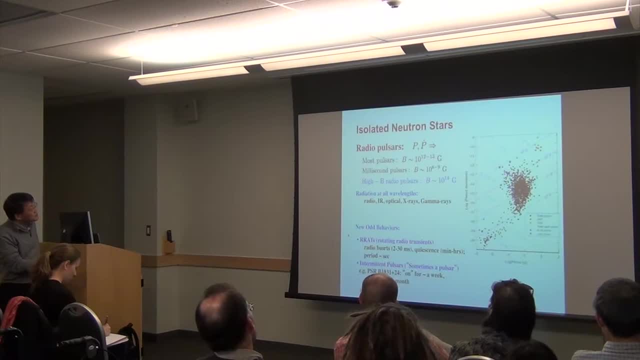 They have a small portion of the pulsar, minority of pulsars, of militant pulsar. They rotate much faster. The spin period, rotation period is about milliseconds, a few milliseconds. They have much lower field than the eight and the nine gauss. 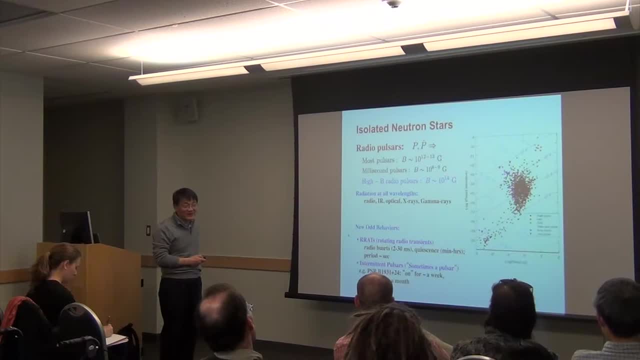 Okay, High and low is relative, but they are. they are pretty high by our standard. That's okay, Okay And right, okay, So they're still pretty large. And then in the last 10 years or so, there is another population of pulsars here. 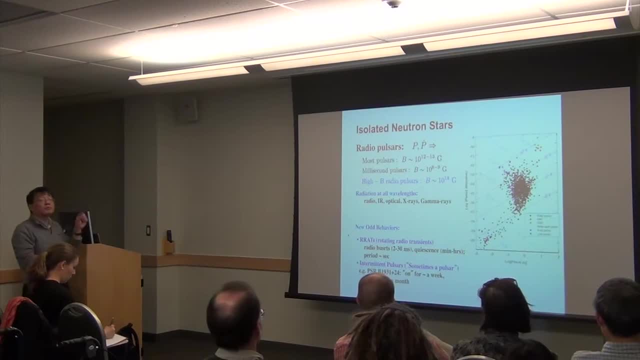 And they. if you do this exercise, measure it with your P and P dot Period and period derivative, You find their P field dipole field is 10 to the 14, gauss even higher. It's very, very high P field. 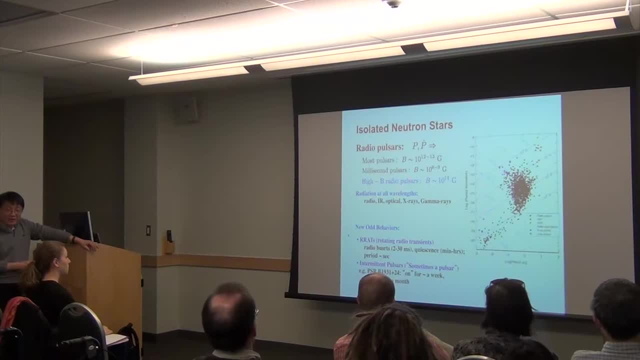 Okay, And of course radio pulsars. you can detect them in radio, but you can also detect them in other wavelengths back, And in fact you can see them in optical infrared X-ray gamma. So they, they, they can also observe other all wide range of electromagnetic magnetic. 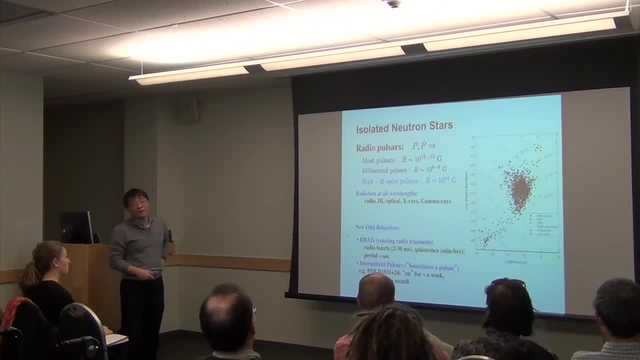 radiation. Okay, So now radio pulsars. astronomers have been studying radio pulsars. for what? for decades now They, it's fair to say we, still don't understand that. there's still a lot of puzzle, very intriguing puzzles. 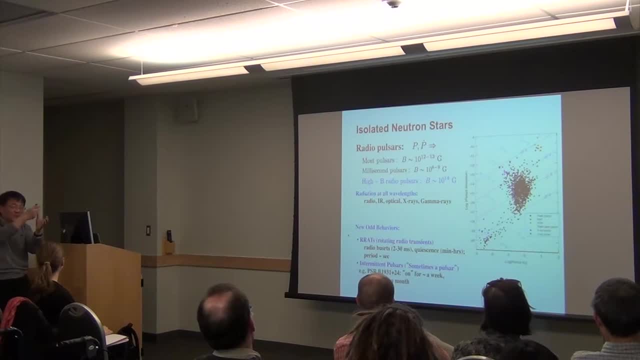 We don't understand them. This clock is simply. it's just something rotating with a big mega field. It's very simple, But if you observe that there are a lot of puzzling things, right, I'm sure people here- Joanna can tell you much more detail- all kinds of complications. 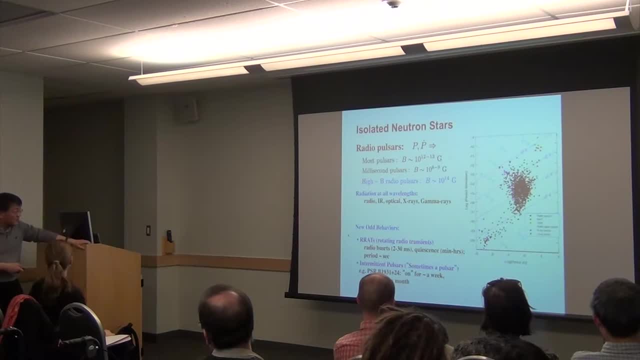 But even even beyond the standard radio pulsar puzzle, there are, there are some new art behavior that was just found in the last recent year, in the last five, ten years or so, For example. let's give you some example. 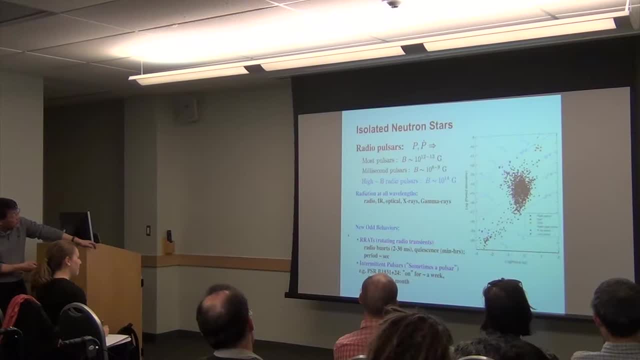 You know this is a rats sort of are rapid rotating, rotating radio transient. So this, this, we don't know what they are, but they most likely are some manifestation of radio pulsars. What happens if you have a pulse lasting for a few milliseconds? then you don't see them. 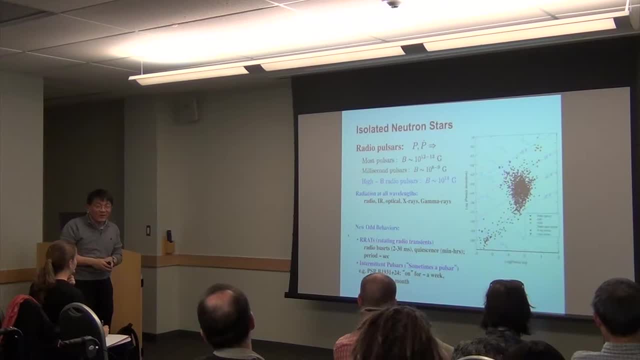 And some other time. it's not a radio pulse. It's not. it's somewhat irregular. It's a radio pulse. Come on, If you do careful data analysis of this pulse survival time, you can decipher the internal period underlying periodicity of this, of this, of this, this, this radio pulse. 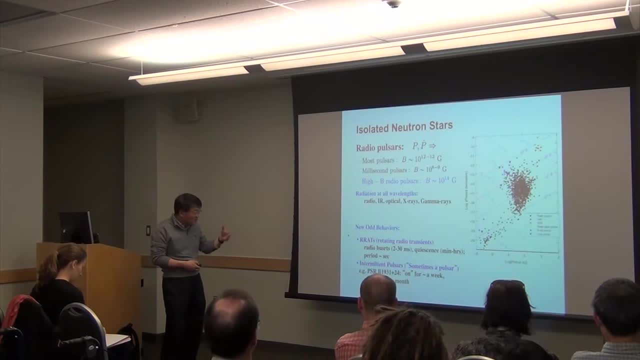 Okay, So this, we think this is also. somehow it's related to the pulsar phenomena. Another one that of great interest here is some is intermittent pulsar or mode changing pulsar, So sometimes the pulsars is. it is a bit more strange. 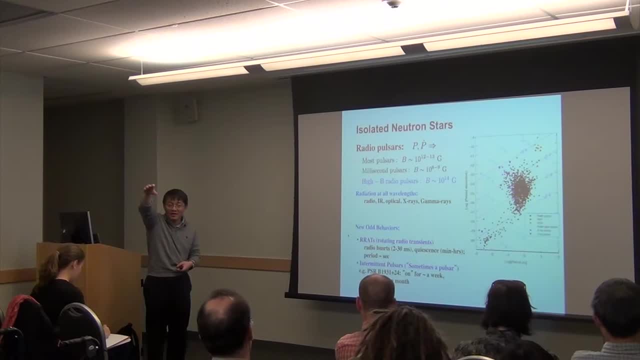 They have. you know pulsar behave very happily, regularly, you know emitting pulses, And then then suddenly within you know, minutes become dark, become quiet, nothing, you don't see anything And for two weeks nothing happened. 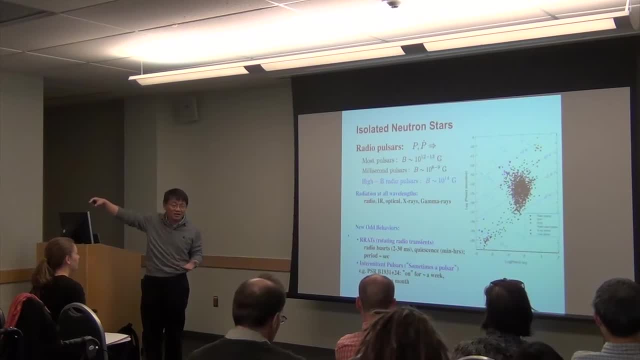 And then, two weeks later, come on again. What the heck is going on? It's very strange. This intermittency is very strange. Okay, So it's a temperamental pulsar. It's just happening here. It's quite a something. something going on. 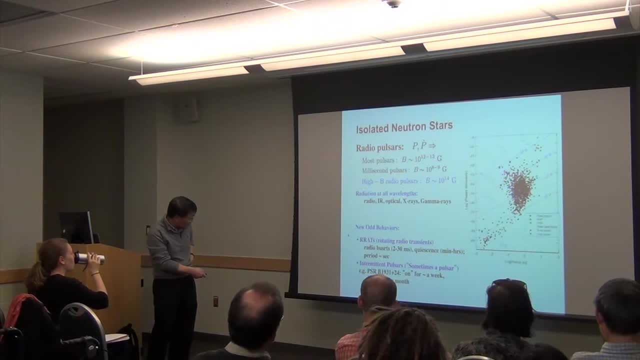 We don't understand what's going on. Okay, And of course, in the some of you, if you pay attention to the news, there's this: so fast radio bursts is another thing that that is happening now, just in the last two. 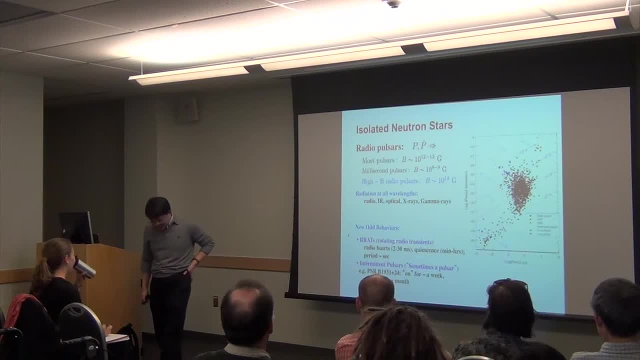 years. A lot, of a lot of news, if you pay attention. a lot of news happened in the. something happened last, last month actually There's a lot of news on this thing. Fast radio bursts. These are again. just you see something that bursting out some kind of you know. 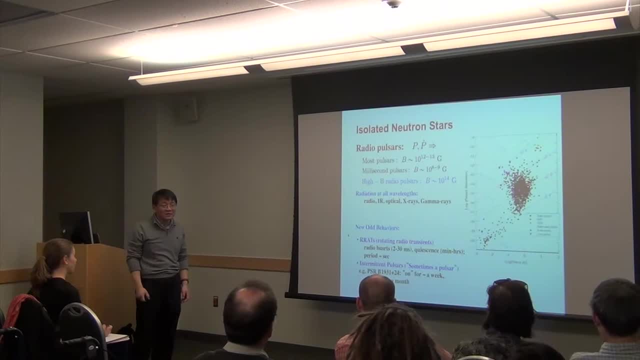 bursting out some pulse. You don't know who they are And they are. they're probably far away because you, by measuring the property of the pulse of LIBOR, you think they are. you think they are from far away, not in the galaxy. 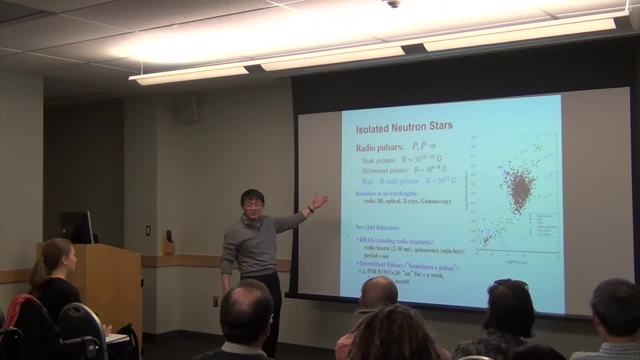 But what they are we don't know. Okay, They may be related to this neutron star phenomenon. Okay, So a lot of puzzles here. So that's the first way an isolated neutron star manifests themselves. Another way that isolated neutron stars can manifest themselves is called magneton. that 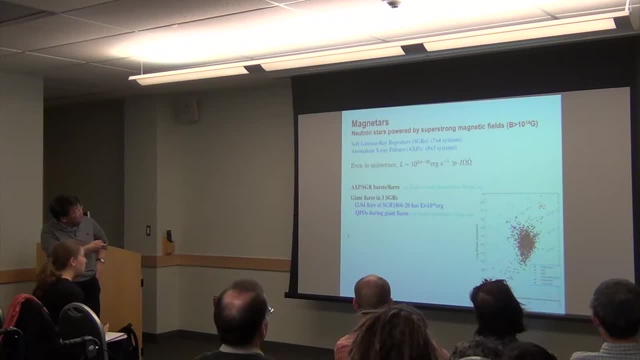 we observed about. you know These are neutron stars powered by a super strong mega field, a field greater than 10 to 14 Gauss, And they- I don't want to go into detail, The buzzword is too used to- you know, people study this kind of thing. they recognize that. 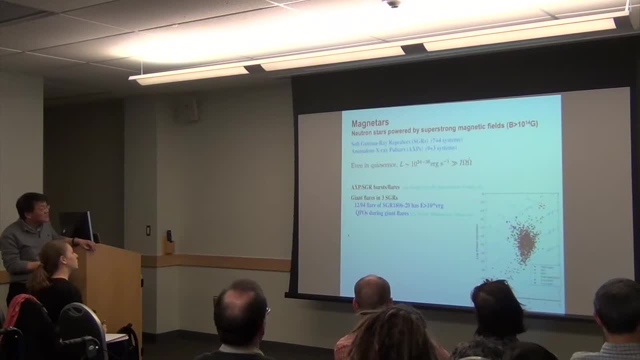 this very strange object called soft gamma repeaters and another kind is called anomalous Epsico source. They don't emit radio emission but they emit X-rays, Some periodicity very strange, very bright And okay. And we now think these are you know, these are you know, these, are you know these? 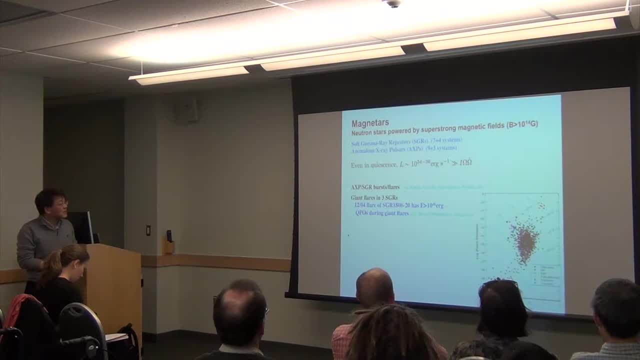 are not magnetic fields. They're magnetic fields And you know we now think these are belong, all belong- to magnetons. And what peculiar about this, all these kind of objects, is that they have field so strong that almost all most of their radiation is powered by the magnetic fields. 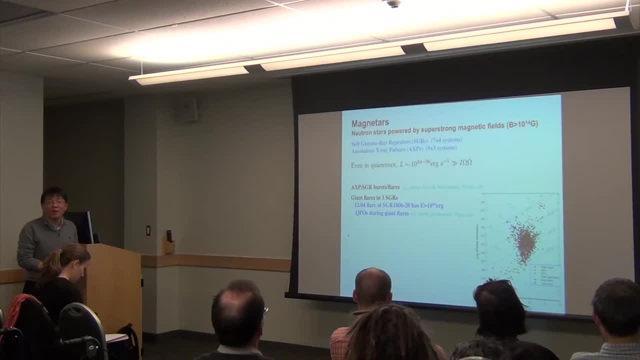 Energy, dissipation of the magnetic field. All the energy that you see ultimately come from the dissipation of the field, magnetic field. Okay, So, for whatever reason, the magnetic field get dissipated and then get transformed, transform in radiation, into radiation. 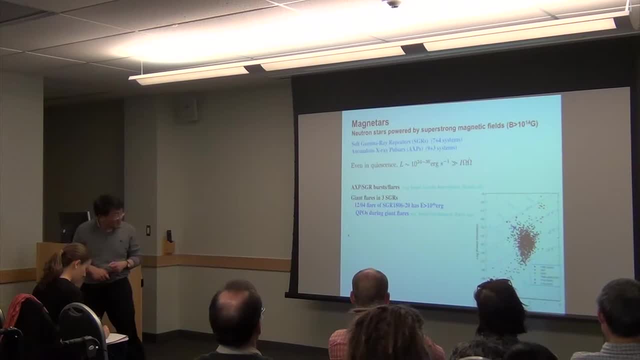 And you know, maybe I'm not wrong- And so these are nanotars. They are also quite temperamental. They have flares, bursts. they don't just sit there quiet, They have starquakes, for example, that are happening. 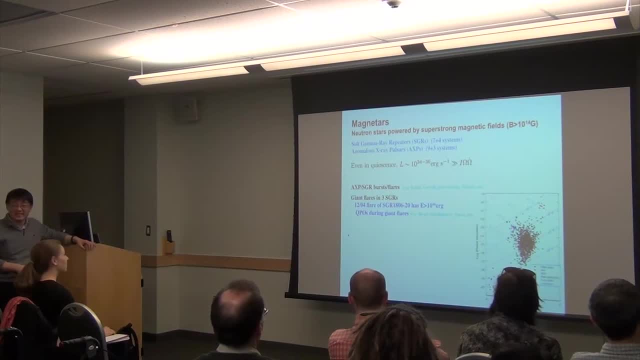 The whole thing is changing in a global way. You can actually see And it actually. some years ago the nanotar outbursts actually affected the communication of the Earth Because the radiation coming from nanotar perturbed the ionosphere of the Earth. 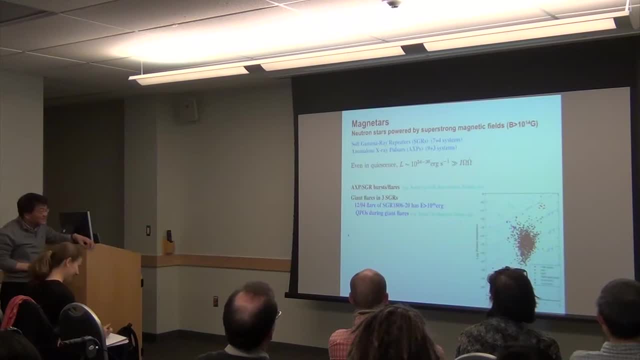 so it affected the communication from the satellite. So this object so far away, thousands of light years away, but yet their radiation, because when they are burst they generate such a large number of energy, They can affect the ionizations of the ionosphere. 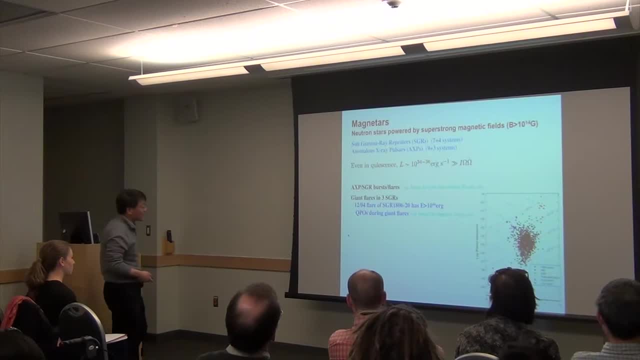 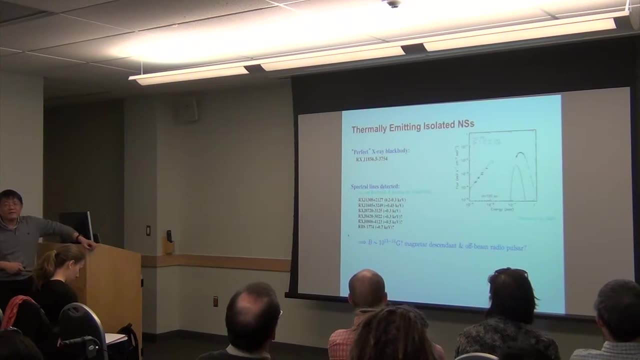 So they have big bursts, flares and a lot of puzzles concerning these nanotars, And then You also have this sort of boring neutron star. just sit there doing nothing, just sit there in space And you don't see their bursts, they're just sitting there. 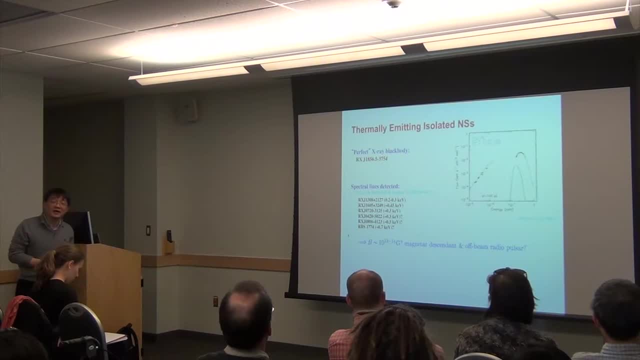 It seems very boring, But they are also quite interesting because they are very hot. These objects are very, very hot. The surface temperature is very hot, Millions of Kelvin. So when they have millions of Kelvin they emit x-rays And if you have very good x-ray telescope, 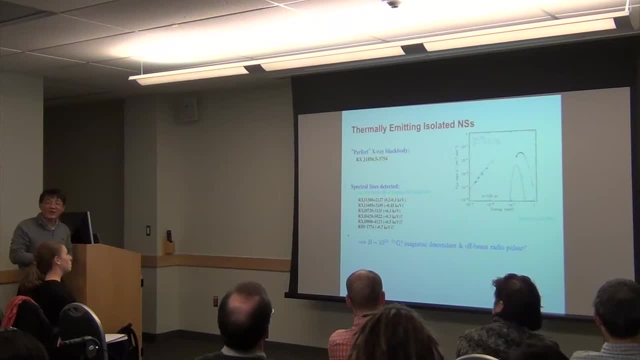 you can actually detect those x-rays, Right? This sounds like very simple, but it's actually very challenging because, if you think about it, this is a very small object very far away. right, You have to be a very sensitive x-ray detector. 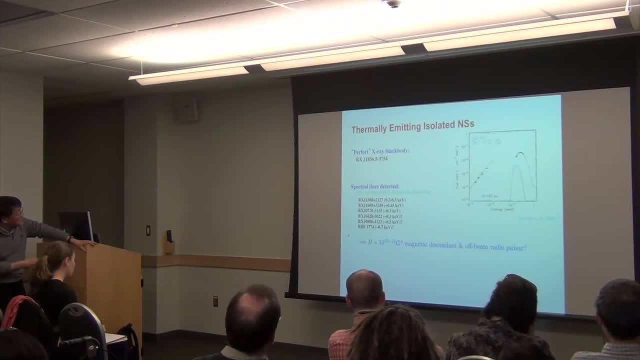 to be able to see those x-rays, But that I haven't seen. And you can even do spectroscopy. You can. sometimes for some systems you can actually see spectral lines, absorption lines, from the system, the line, And that I haven't seen. 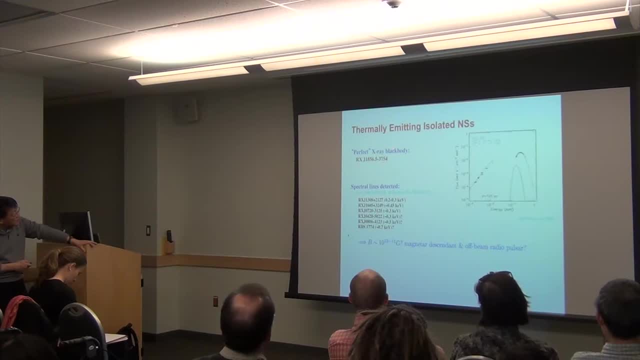 And in one object. I want to single out this particular object which is very intriguing because it's actually a very good. if you look at the, you have very good x-ray telescope. you look at this thing, you find the x-ray radiation. 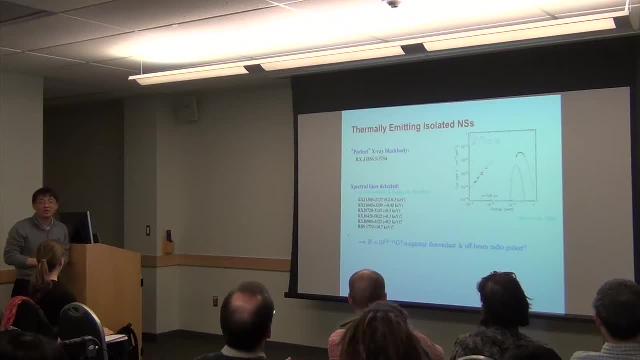 it's almost a perfect black-body radiation. Textbook level: textbook level black-body radiation. This is the second best black-body in the universe. The best one is anybody know. Big Bang, Big Bang, Big Bang produced the best black-body. 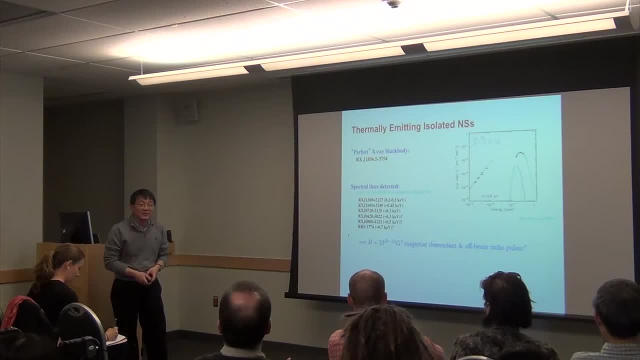 And this is the second best black-body. It's not easy to produce black-body because to produce black-body you have to have a perfect condition. You have to imagine the radiation will matter perfectly in time with each other. It's very difficult. 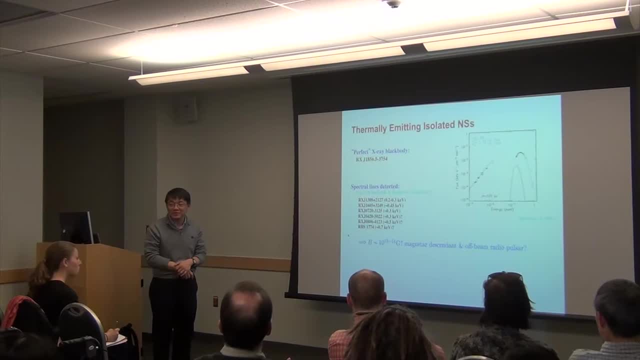 And the sound is not black-body radiation We talked about. when you learn physics, you learn black-body radiation. That is not easy to see in nature, a real black-body, and this is very good. So I come back to this a bit later. 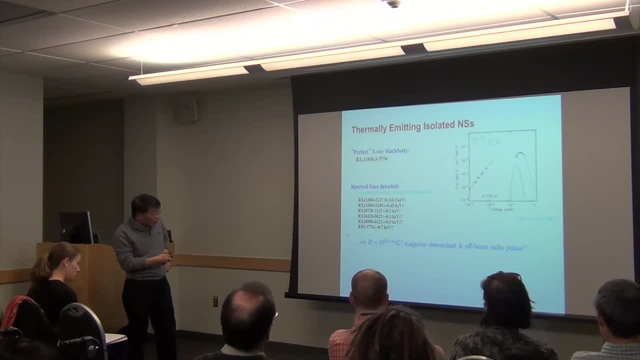 So now some of these post-based objects also have rotation p and p-dot measured. So again doing that exercise, assuming the slope, the p-dot is due to the net dipole radiation, You can infer the b field. They are very high, these 314-dots. 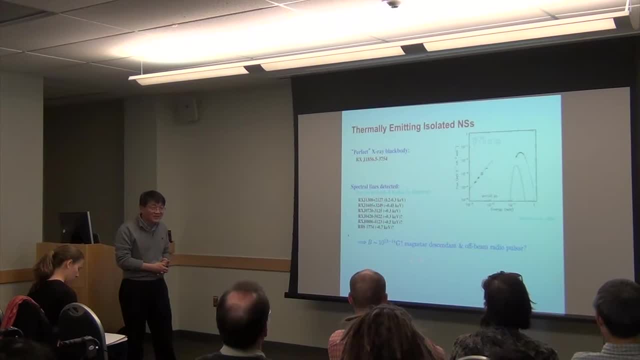 So maybe they are the descendant of megatons, Or maybe they are radio-posons. We just don't see them. Maybe they are just sitting there with the radio beams pointing away from us. we don't see them, so we don't know. i put the question mark here. we don't really know, so that's. 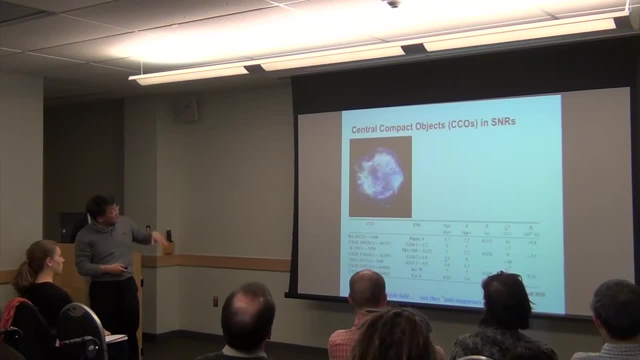 another manifestation of neutron stars. and then finally we have the so-called cco central compact object in supernova remnant. so i mentioned supernova explosion earlier on. when you have explosion, this explosion is not into the vacuum, it's into interstellar medium. this explosion leave behind a remnant emitting all kinds of radiation. so inside of this supernova remnant, 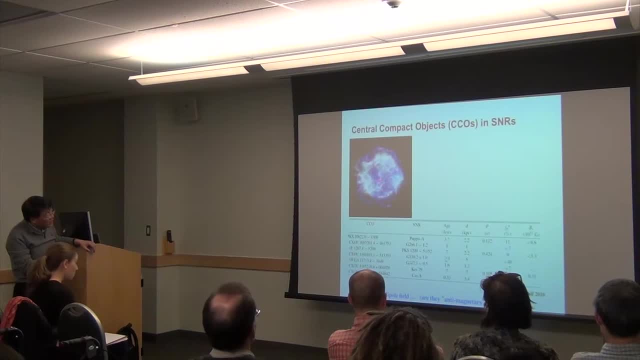 at the center. there's a point here as well. this point is actually a neutron star. people have detected with a big, powerful telescope, right? so there are about a half dozen, also more than now, but at this time their point source have been detected at the center of supernova running. 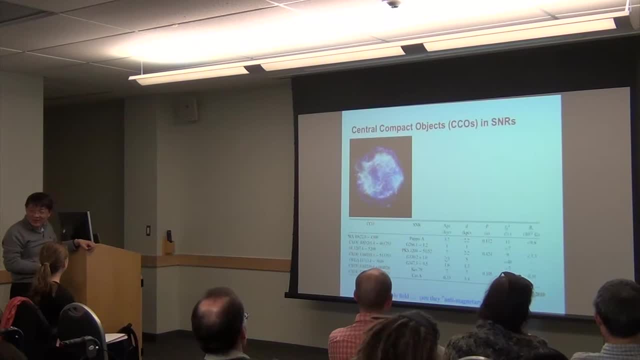 right, and this, this, this thing, that certainly neutron star, most likely, and again you can measure the period and period derivative- infer their magnetic field, but strangely, the dipole field of this object is relatively small, you know, probably 11 gauss or less. very strange, right, because these 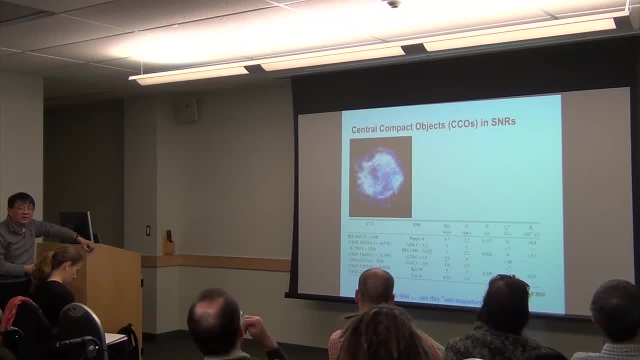 are? these neutrons are embedded in the supernova remnant, so they are very young and yet their field some points lower than the typical value. you know, most radio posts are a little tall girls. this change, right. if that one: you get older you feel stronger, that's usually you think decay, right. 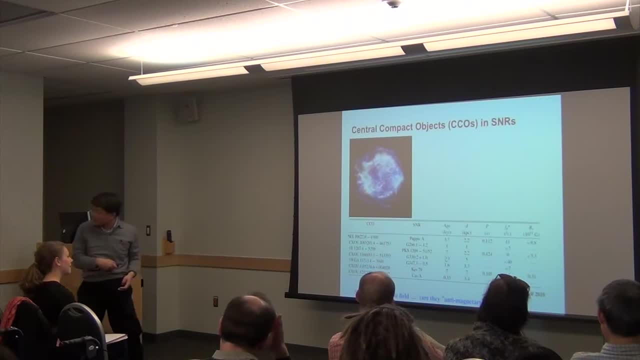 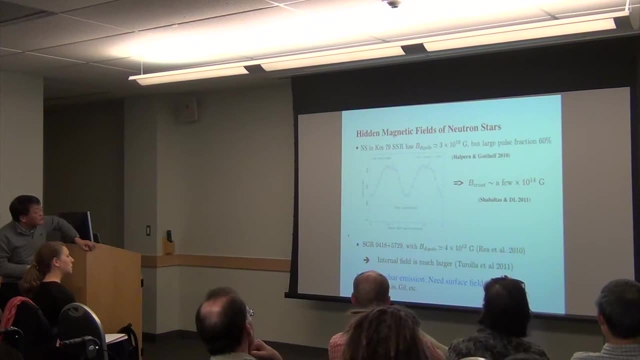 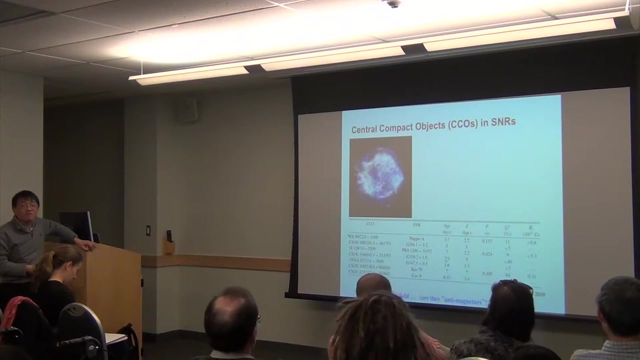 but this gets longer, this change, okay, we don't know what's going on. that's the answer. first thing at this point, okay, um, now i want to have a comment on the magnetic fields of neutron sun. emphasize everything i said when i say magnetic field: right, these are the dipole field inferred. not direct measurement right. you measure period and period derivative and you assume dipole radiation. you get a dipole field right and there is evidence that the neutron stomach and field is much stronger than the dipole field. there may be hidden magnetic field inside the neutron stars. i. 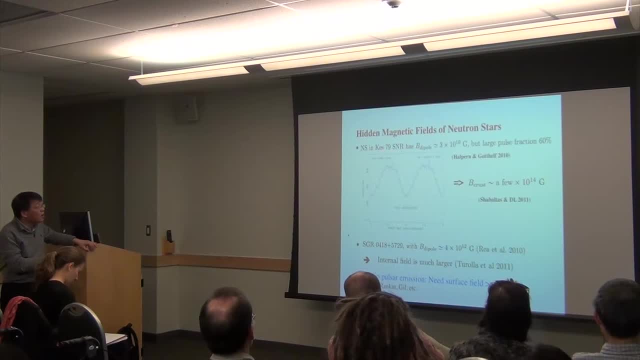 don't want to go into detail. right, and for example, this particular object, the dipole field, is 10 to 10 gauss. but they're the reason to believe that inside the neutron star, the b field, or near the reach, near the surface of the neutron star, the b field is much larger, with 10 to 14 gauss. okay, 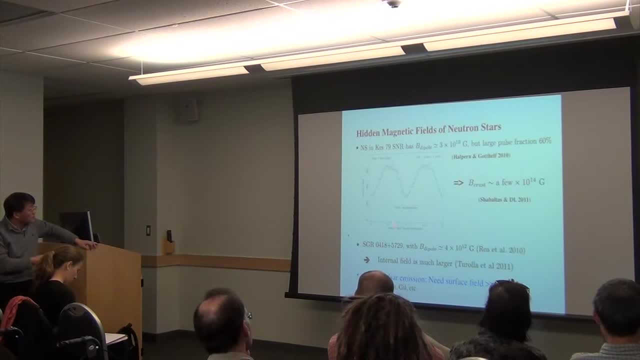 and uh, there are several kind of systems where you know this is this particular system. there are many power and this, this type of field, normal, but yet in the magneton. so it's very strange. okay, and from radio post observation there's also some evidence factor to explain some of the radio post. 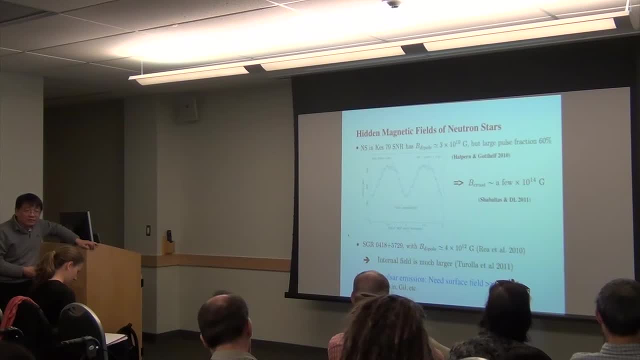 observation, you really need a surface field much greater than the dipole field, so this is actually very important. i think we'll try to really infer what is the true negative field of the neutron star, and that's very important. okay, so that's the summary. the inventory of isolated 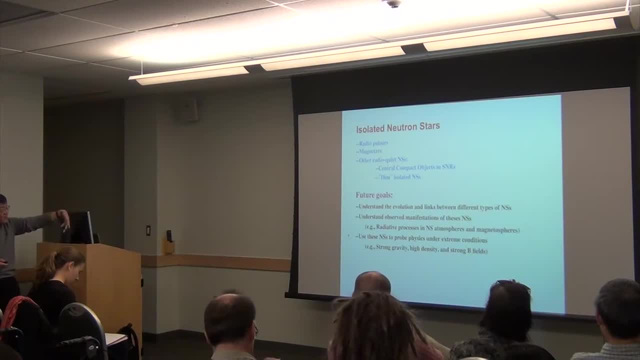 neutron stars. we have radio, post source, magneton, radio, quiet, so they're all quite different. so what's the? what do we? why do we care? well, we care. what's the goal of doing this kind of thing? well, clearly, we want to understand what's the link, connection between these different manifestations. 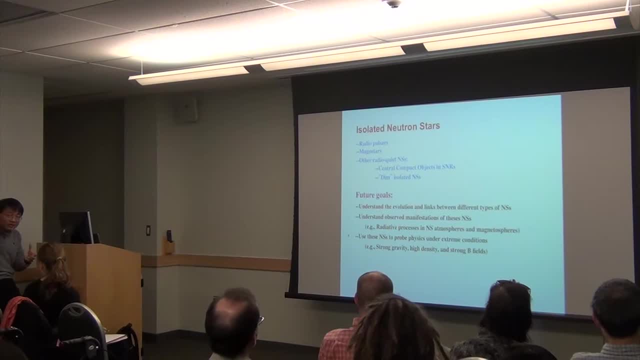 of neutron stars, right, well, how they are related to each other, are they dependent of one to the other? how they evolve? but why you have this different manifestation, right? what? what tells me the key property of the neutron star? and we want to understand, for example, why you are in the radiative. you know how they manifest themselves. 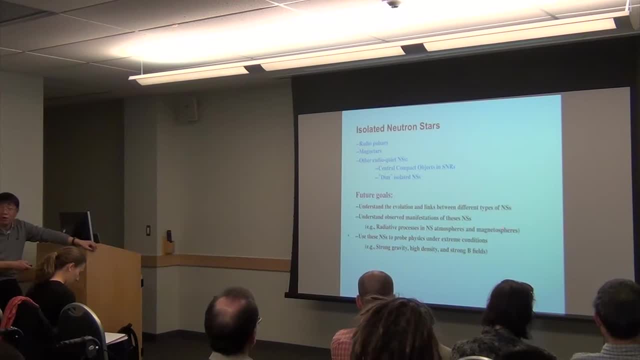 right the radiating processes in the neutron star atmosphere and also in the focal magnetic field. what's going on? why the you have this burst of radiation pulse coming out right? what's the emission mechanism? that's a long-standing question. that's very important. and then and then you can also, of course, use neutrons i already alluded to. 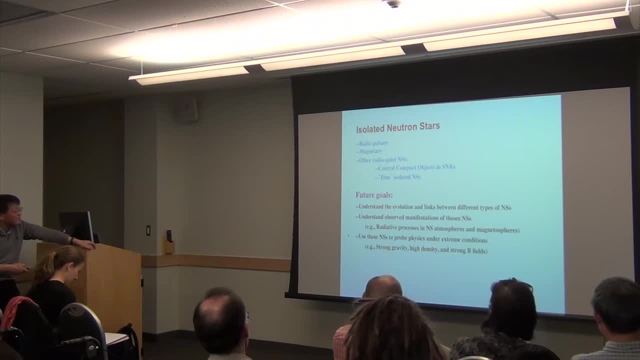 right that you can use the new transfer to probe the physics under very extreme conditions. right, neutrons have very strong gravity, very high density, strongly confusing. by looking at some of the property of these neutron stars we can learn something about probe the physical and very extreme conditions. so now let me give you some example. with these last points, right, how do we? what kind? 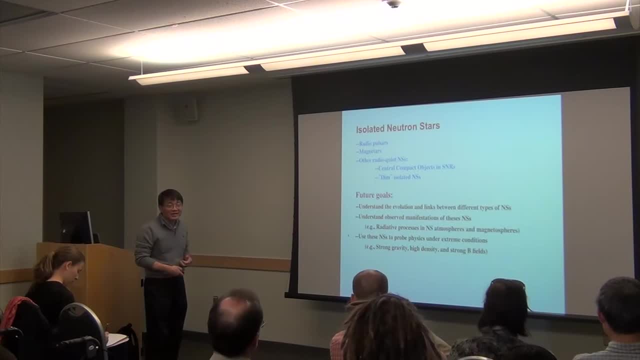 of extreme physics we can expect in such a strong, such exotic neutron star. right, so this? of course, there are many, many examples. i could spend hours talking about this, say, i'm going to give you two examples, right, two examples: the probing between physics of neutral stars. the first one: 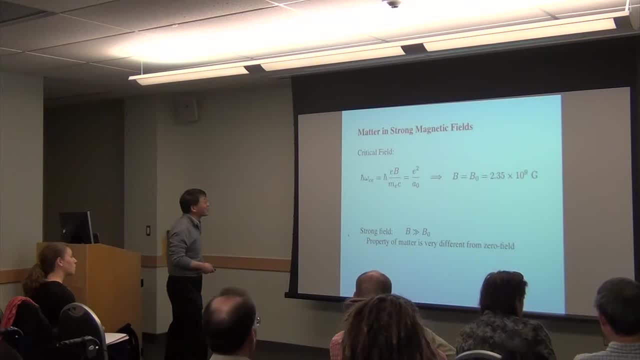 so, if you feel, between two examples, the first one let me. i want to talk about data in very strong magnetic field, right, uh, so we have such such a strong magnetic fields, what's the behavior of matter on neutron star? now you say, well, you transfer their nuclear density into the 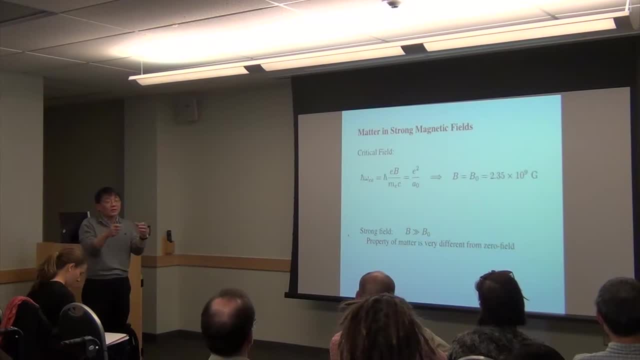 very high density. But remember it's true in the central region the density is very high, or the bulk regions are high, but near the surface the density is low. right When you go to the surface the density is quite low. so there's a matter there also. 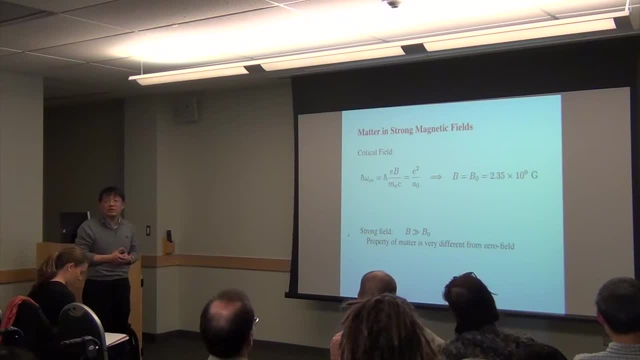 right, You could have atoms, right? You can just ask a general question: what's the behavior of atoms and molecules and condensed matter in such a strong matter field? because this is the kind of field that we don't encounter in laboratory, You cannot create in laboratory. 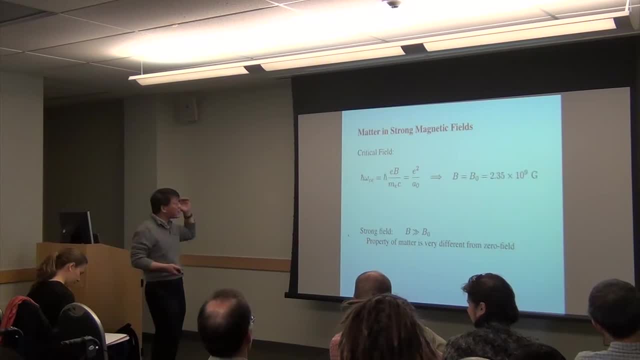 So you can ask what's going to happen. what's happened to the atom right? So the first question you should, before you say strong matter field, you want to ask what is strong by strong. One of the important things when you study actual physics is: you learn that everything. 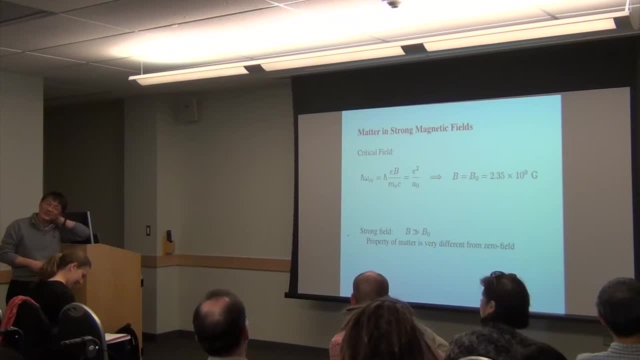 is relative. right When you say strong, how strong? how strong is strong, by what standard? right. So when you study atomic physics, property of matter, the energy scale you're dealing with is the energy scale. It's a ball, ball ball: energy E squared over ball radius, basically. 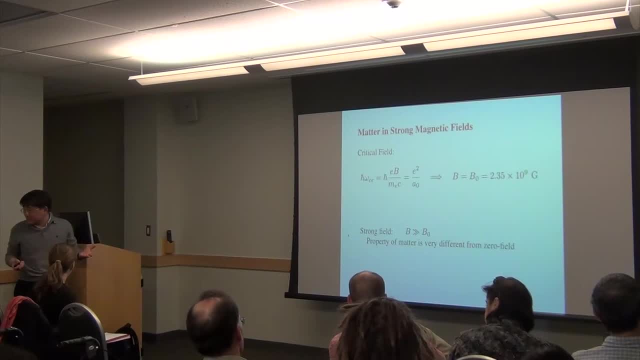 E squared over the ball radius. that's the scale for atomic physics. right, All the energy level of atoms, condensed matter that has this energy scale right, E squared over ball radius. So two Rydberg two times 13.6 electron volt right. 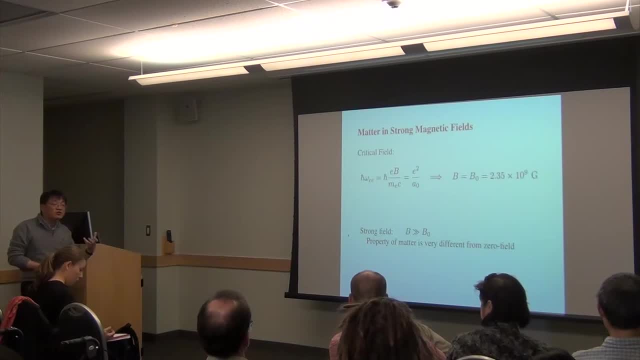 So when you have magnetic fields, the energy scale you're dealing with is the so-called energy. What this is is that you know when you put the energy scale, you're dealing with the energy scale. You know when you put the electron in the magnetic field, it has gyration, classical. 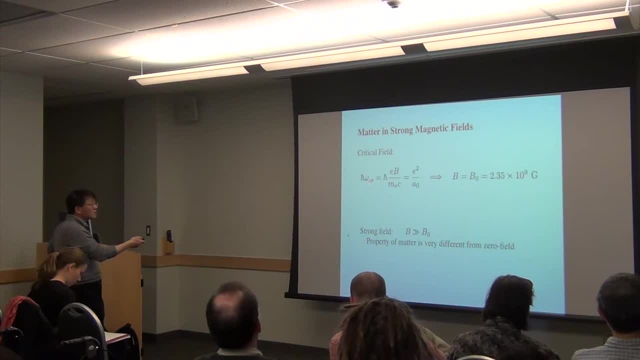 electromagnetism and gyration. that's called cyclotron energy. right, When you quantize that motion, when you put in quantum mechanics, that gyration is quantized, It's called Landau level and that gives you an energy scale: h bar times the gyro radius. 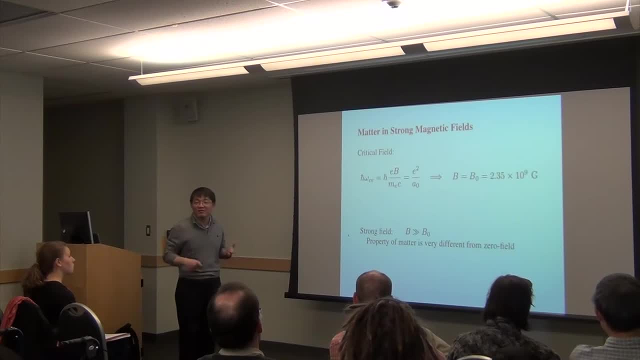 okay, So that's the energy scale associated with the magnetic field. okay, So when we say how strong is strong, if you want to study, you know to what extent is strong And, in the same way, why is it strong? 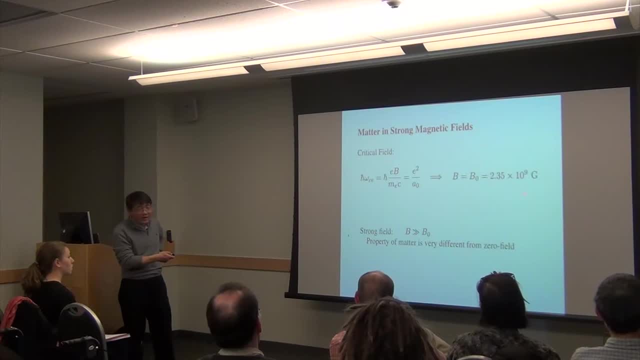 Why can't B field affect atomic structure? This is a critical field you're dealing with, right. So equating the cyclotron energy to the ball energy, atomic energy- gave you critical field, right. So what this says is that if you have B field, much less than this- then the Coulomb force. 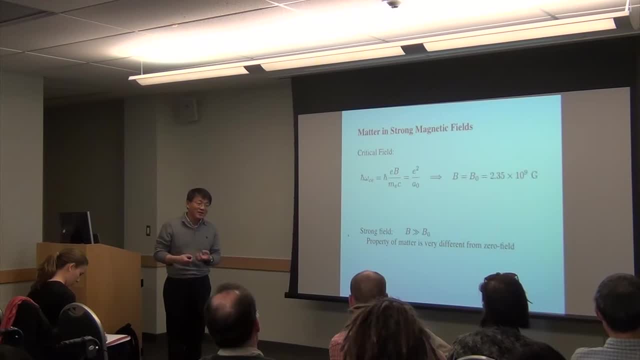 inside the atom much is dominant, right. Magnetic force is a perturbation. You can do V-min effect, V-min force, V-min effect splitting. if you study atomic physics you learn Z-minus splitting, right. You can do Z-minus splitting that kind of things in the regime when B is much less than B0, right. 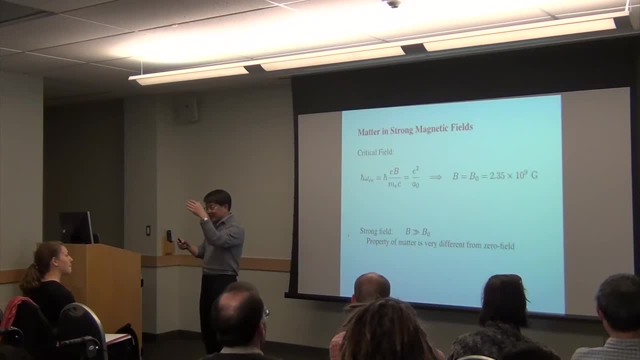 So everything you learn in textbook atomic physics is Z-minus splitting. if you are in the weak field regime in the sense that B is less than B, is good for that. Now, in neutral star- I just told you- the B field typically is 10 to the 12th cos or higher. 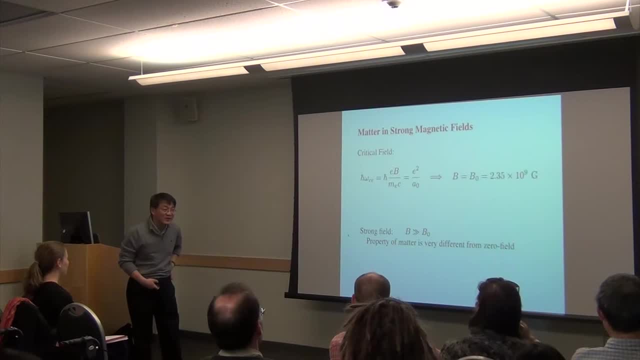 But we are in the opposite regime, right That would? B is much greater than B0. So in that regime you cannot do Z-minus splitting right, Because the B field magnetic force is not perturbation. In other words, if you put an electron beside a proton, the magnetic force acting on the electron due to the external field is much greater than the Coulomb force. 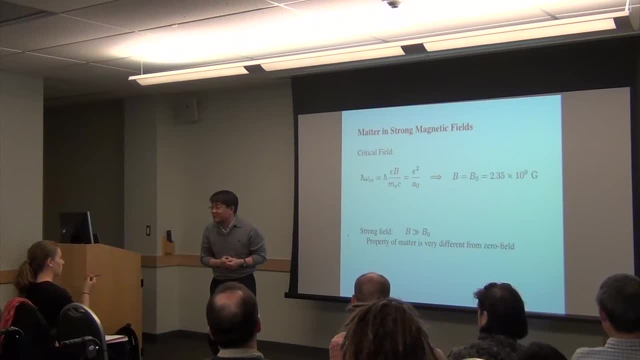 So you should do the other thing. Coulomb force is a perturbation, right? It's the other way, Right? So, not surprisingly, in such a strong field regime, this regime, the property of matter would be very different from the zero field case. 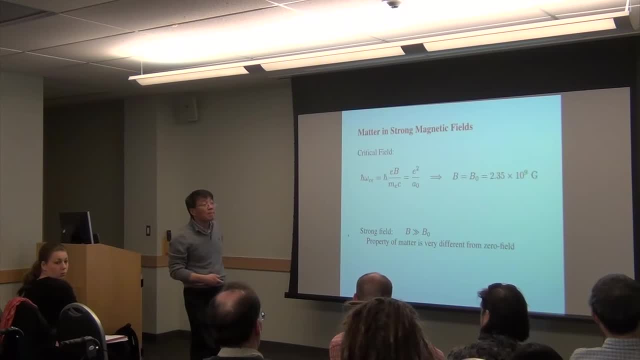 This is orbital field, right? Sorry, This is orbital component of the field, right? I didn't understand why you distinguish between Z-minus and strong field, right? Yeah, what I'm saying is when you do. All I'm saying is when you learn. 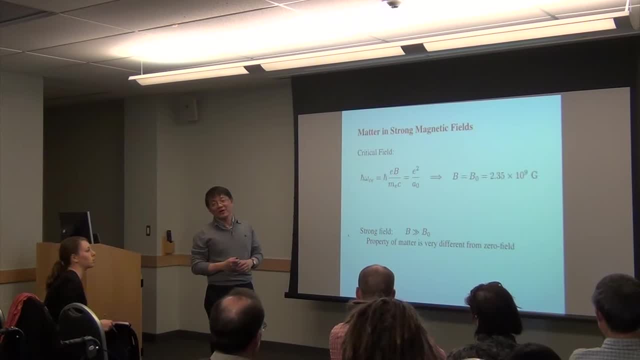 It depends what it's coupled to. That's right. yeah, All I'm saying is, when you do atomic physics, you probably learn Z-minus splitting. You have atomic energy level, you have. add a small field, you have splitting. All that language is based on perturbative theory. 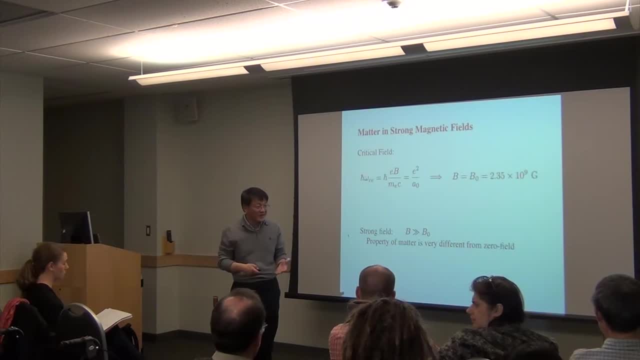 You're thinking the B field is small perturbation. That's right, right. The orbital and spin splitting coexist at the same time. That's right. spin also, yes, The spin part of the B field is small, and the spin part of the energy is also small, right. 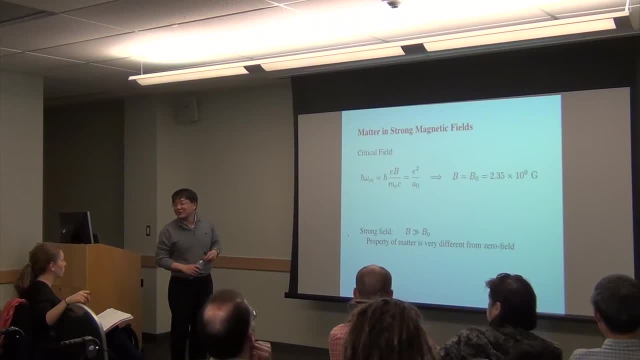 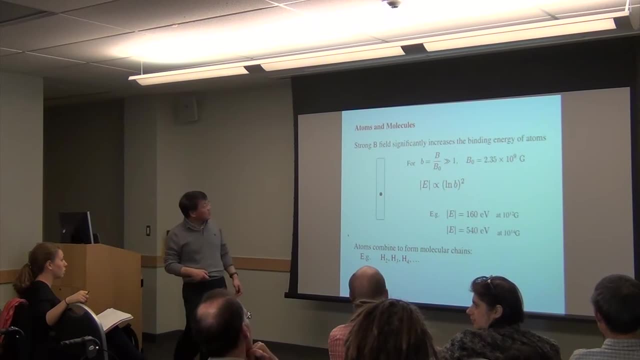 But here we are in the opposite regime. The B field is much larger, right, Okay? So as a result, for example, the atoms are very different from the zero field. For example, hydrogen atom, A proton, one proton. 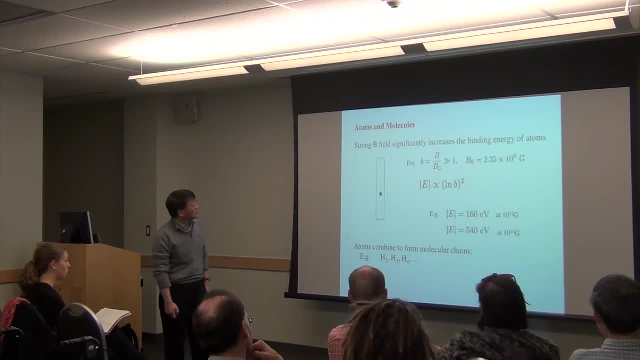 Electron. one electron Become elongated right. The atom is actually become a cylinder. Not so surprising, because you know it's Transfers to the B field is constrained. The electron is. The motion of electron is constrained by the B field. 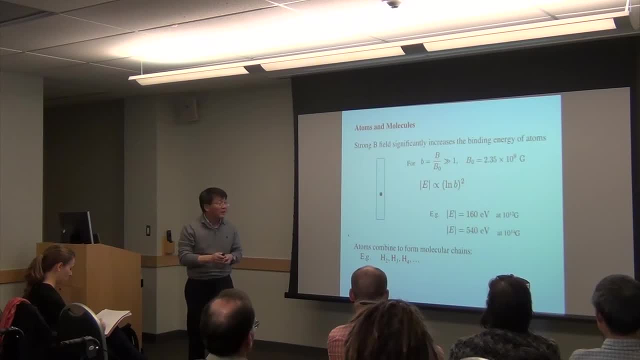 It cannot move a lot. It's just confined by the B field. But along the field, along the field direction, it's constrained by the weaker coolant field, So it's elongated. So the whole thing is very squeezed in the very 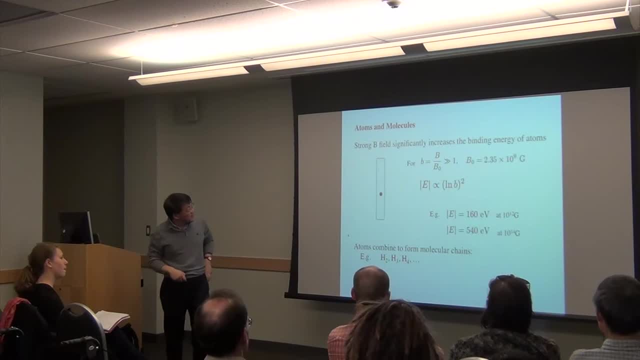 Become a cylinder right And then elongated right. And so if you do calculate it, you find that the B field, the binding energy of hydrogen atom, increases at the bulk of B. This little B is B divided by B, the critical value. Increases at this way, right, For example, the ground state, hydrogen atom energy, binding energy, become 160 electron volt. We have 10 to 12 Gauss as opposed to 13.6 electron volt, right, 13.6, 13.. 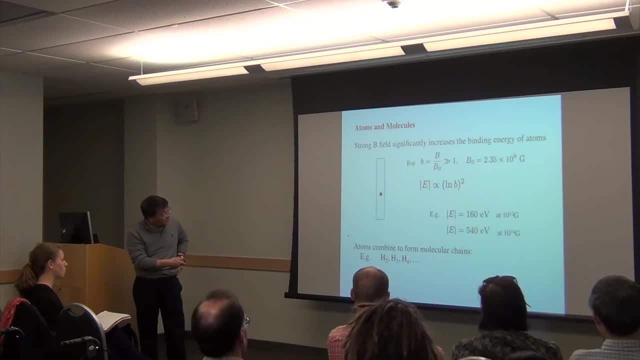 Right. If you go to 10 to 14 Gauss, the binding energy of hydrogen atom in the ground state become half KED. So it's much larger Than the 13.6 that you are used to, right, Okay? 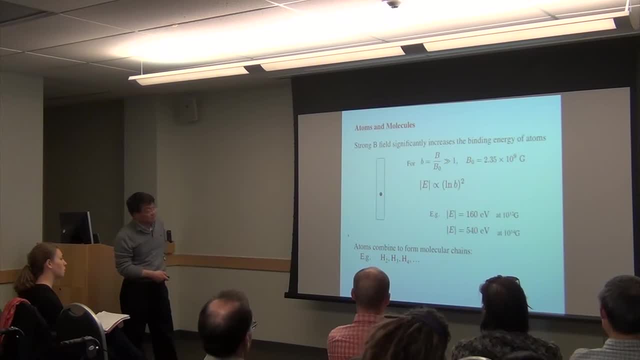 And so binding energy is greatly increased And the atoms can combine into molecules and molecular chains. You can add atoms together along the chain By covalent bonding. you can form molecular chain long chains And you can put chains together into a condensed matter. three-dimensional condensed matter. 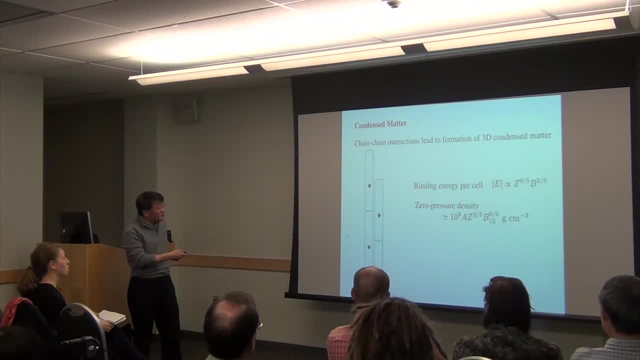 And this can be, You can estimate the energy scale of the scaling of this thing. And Right So this condensed matter. they are squeezed by the magnetic field, Yeah, Right So, even at zero pressure, even if you don't squeeze them, if you don't exert external pressure to do it, they have. zero pressure density is about a thousand gram per cubic centimeter. Right, Depending on the field strength, You can put 10 to 12 Gauss field. The zero pressure density of a solid is about a thousand gram per cubic centimeter. 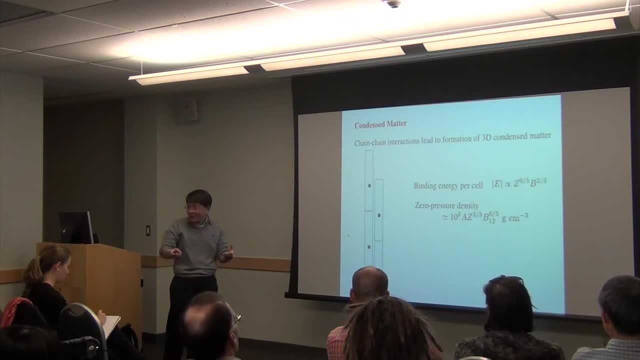 As opposed to one. a few gram per cubic centimeter. Right, All the condensed matter we see in this room, myself included condensed matter, everything in density- is about a few gram per cubic centimeter. What I'm saying here is: you have 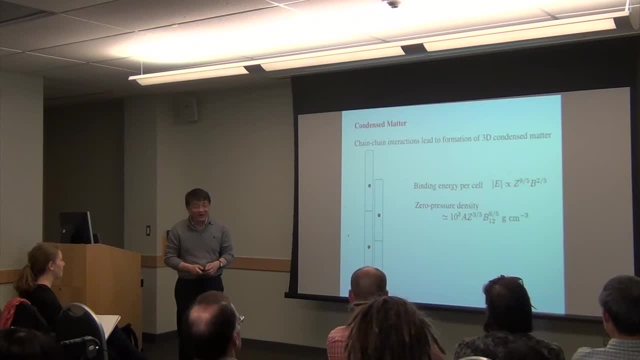 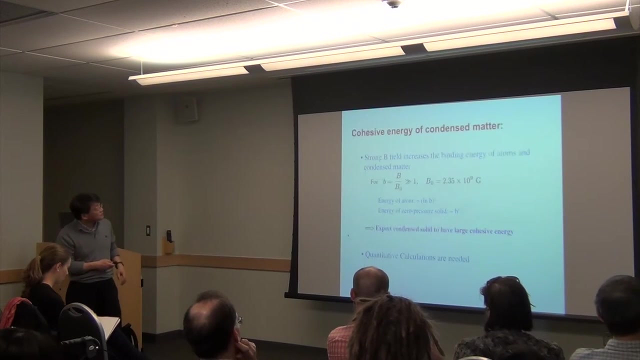 When you put this thing in the strong magnetic field of 10 to 12 Gauss or higher, the zero pressure density, condensation density, is much higher, Simply because magnetic field help confine it, squeeze it. Okay, And So it's quite different. 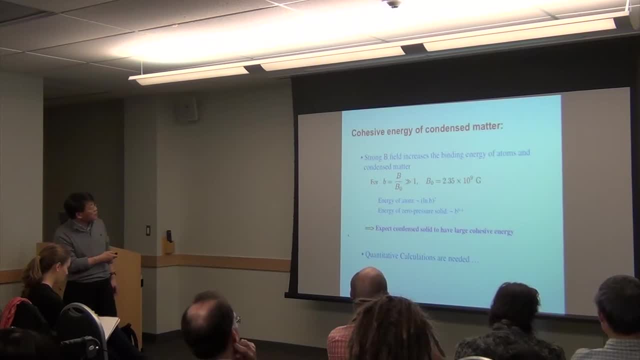 And So So I told you that strong field increase the binding energy of atom molecule condensed matter. The key thing. so I'll repeat right, Basically this: How the B field scale depends on related to B zero Right. 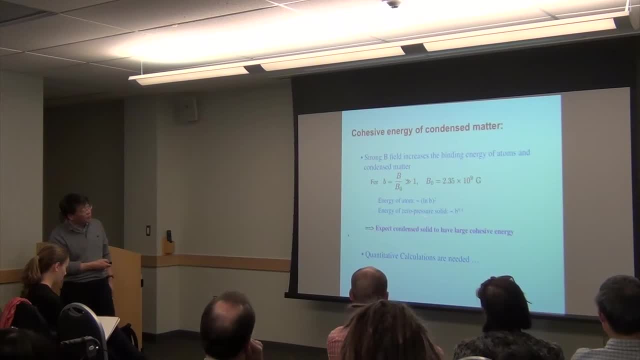 The energy of the atom scale is log B squared: The energy of zero pressure density, The energy of zero pressure binding energy of solid scale B to the. I'll divide this and scale the power law function of B So you can see that you have. 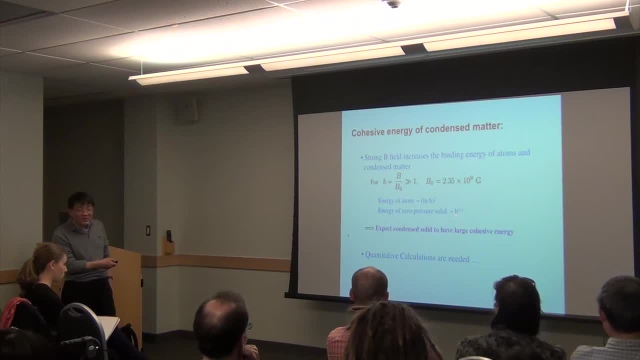 The B field increases. This power law will eventually become very important. So the difference between the binding energy of atom and energy of zero pressure solid is what we call cohesive energy. How cohesive the solid is Right If you want to have a solid. 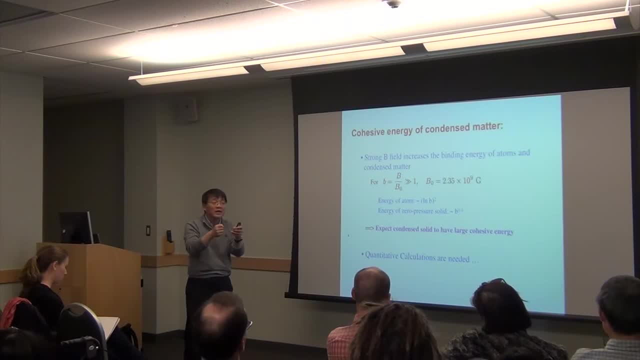 this must have a finite cohesive energy. So how much energy you take to break up a solid, basically, Okay. So So you're comparing this difference between this, This energy of individual atoms, and energy of A unit of atoms sitting in the solid. 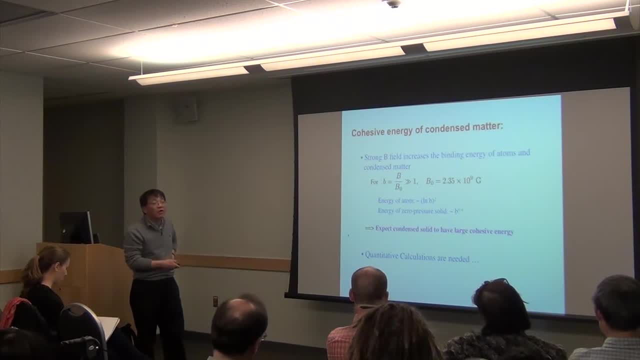 Right. So to give, To really determine the cohesive property of the solid, how strong the solid is, you have to do both, say calculate engine atoms and calculate energy of solid. Okay, And this, To do this you have to do quantitative calculation. 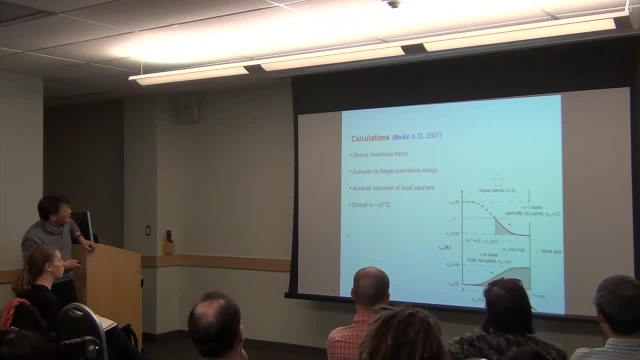 So we've done this- actually a couple years ago, some years ago, Right- And we've used some density functional theory- Some of the experts may know what it is, I don't want to go into detail- And we've improved the accurate exchange correlation energy. 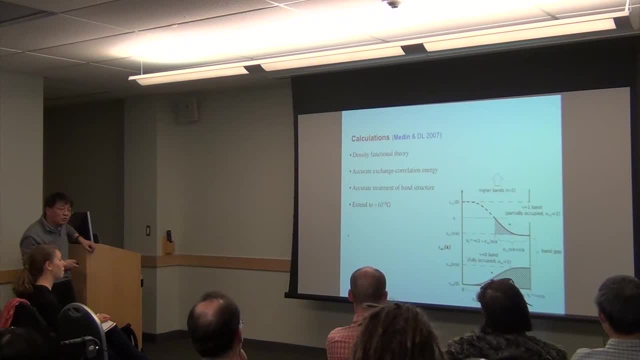 And we had to do the band structure. In this case the band structure is one-dimensional, So actually It's actually easier than the Than terrestrial solid, Because terrestrial solid is three-dimensional. Here it's one-dimensional, So actually in some sense it's easier. 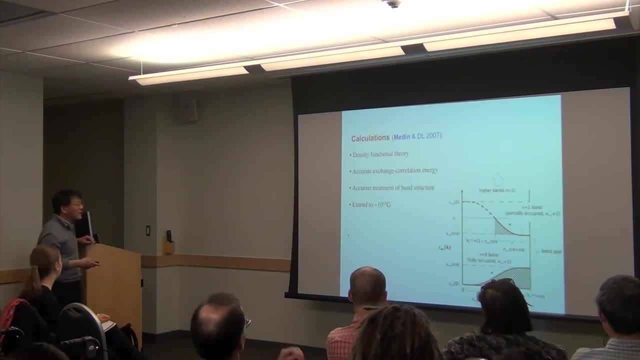 It's more erotic, but it actually is somewhat easier. Okay, So we did some serious condensed matter physics calculation. So here's the result: Right? What we find is that cohesive energy is a function of field strength. Right, For example, for iron it's solid. 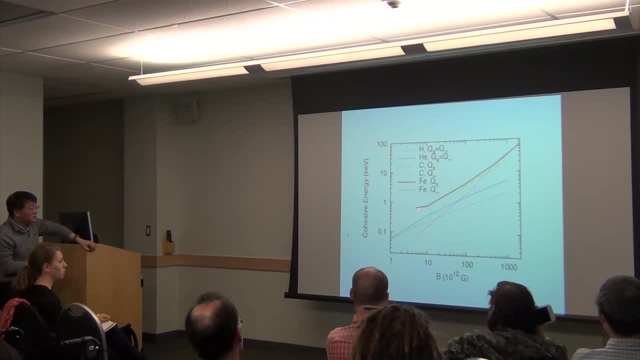 It's iron Right Solid line. You can see. you know the cohesive energy becomes a Ke. You know, at 10 to the 13th Gauss it's a KeV. If you keep increasing the field it can become. you know hundreds of. 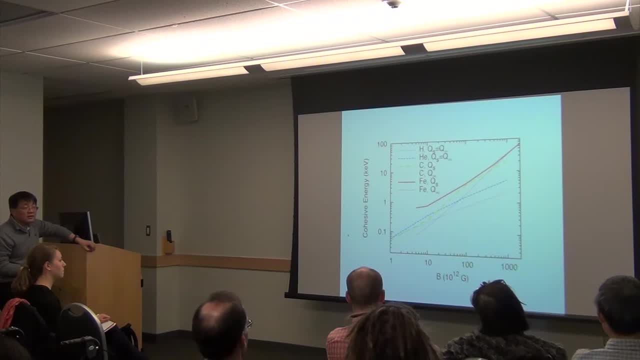 Thousands Tens of KeV. By contrast, the cohesive energy of the normal solid in terrestrial On Earth it's about one electron volt. You know a fractional electron volt, a three electron volt. So here we're dealing with cohesive energy of kiloelectron volts. 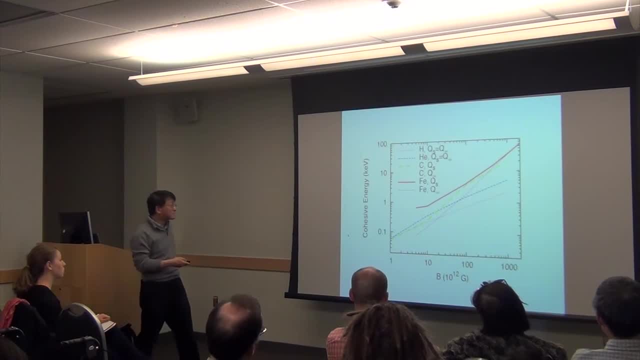 Or higher, Depending on the field strength. Okay, Now you say, well, why do we care? Why do I bother with this thing? Why do you care? Why do we do it? Well, it's fun to calculate all the different forms of terrestrial. Why do you care? We do care because they're actually implications After physical implications That can affect operations. Okay, So let me give you the example. The first example is that I mentioned earlier that this particular, One particular neutron star I mentioned earlier, this one had the perfect second best black. 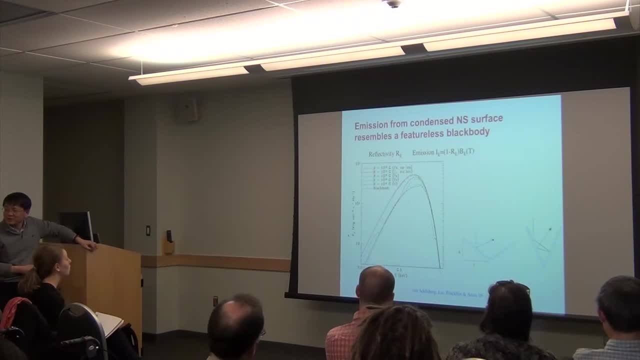 body in the universe. I told you that it's very difficult to In the normal storm. the atmosphere, like the sun, the earth has an atmosphere. the emission, the radiation from the sun or from the earth is not black body. it has all these bumps, wiggles. 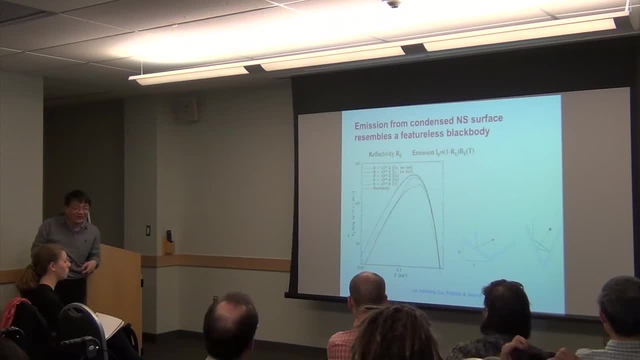 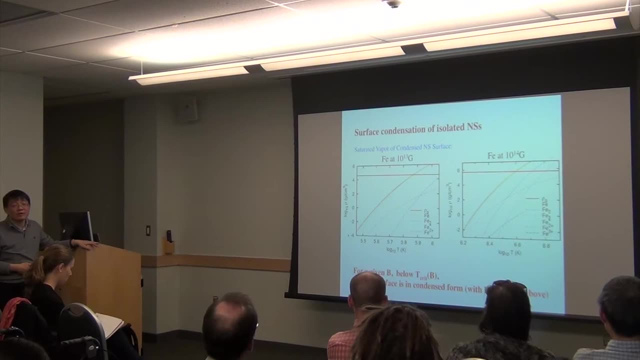 But these neutrons are very clean, perfect black body. so what's happening? So one possibility is that these neutrons happen to be very cold and also have very strong magnetic field. So the outermost layer of the star is all condensed into a shiny solid. 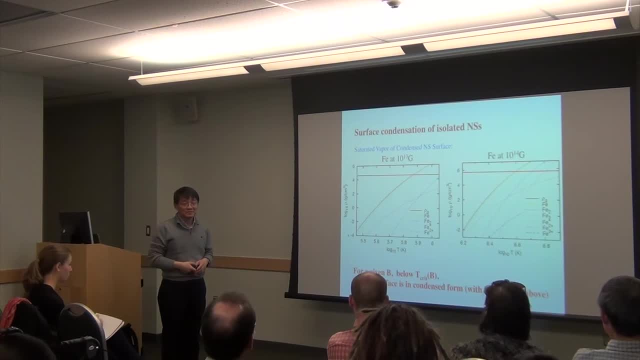 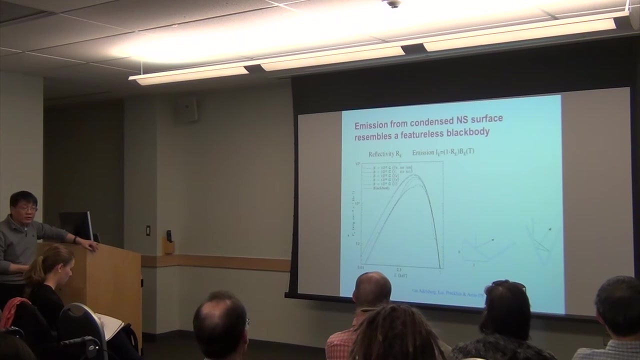 All condensed, no gas above it, Just bare shiny metal. And despite the fact that the temperature is 36 Kelvin, the B field is very high. so it's all condensed, So So that If you have radiation for a condensed material, it turns out you can make such a condensation, you can make an almost perfect. 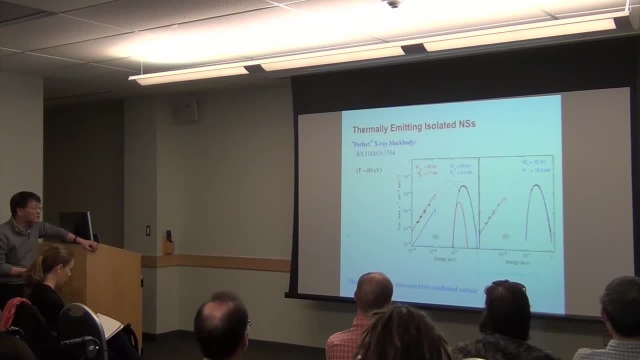 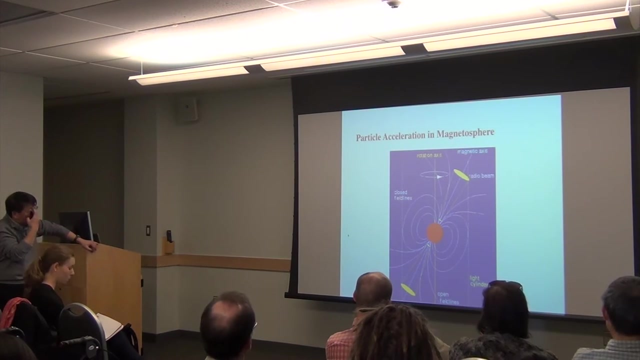 Under some conditions you can make a very good black body emission. So this: maybe you have a condensation that helps explain this almost perfect black body radiation of this particular object. Another implication: why do we care about this condensation? It has to do with the complicated problem of pulsar radiation. 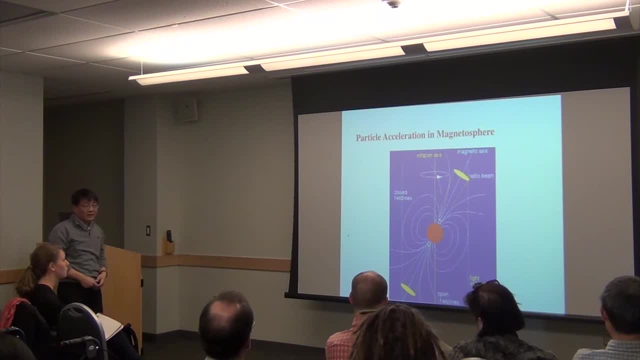 So pulsar, I told you earlier, emits radio waves right Now. it's a very complicated process but roughly speaking, to emit radio waves you have to have particle acceleration. You have to have particle. It can accelerate to very high energy to emit radio waves right. 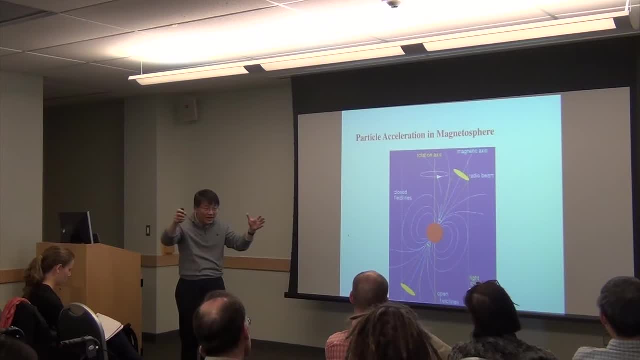 And you have to have a so-called magnetosphere outside the neutron star and they Some way that they can accelerate particle, can accelerate it and Right, And emitting beams, beam radiation. This is a very simplified picture Because we don't have time to go into this. 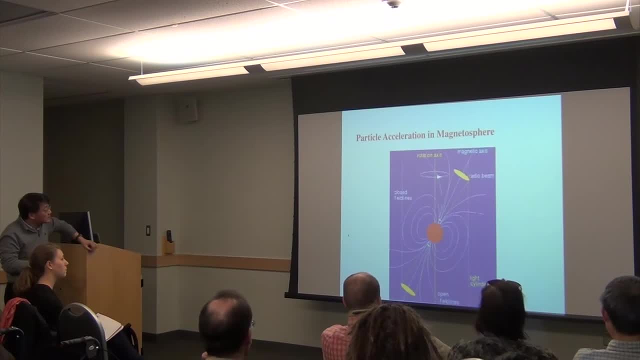 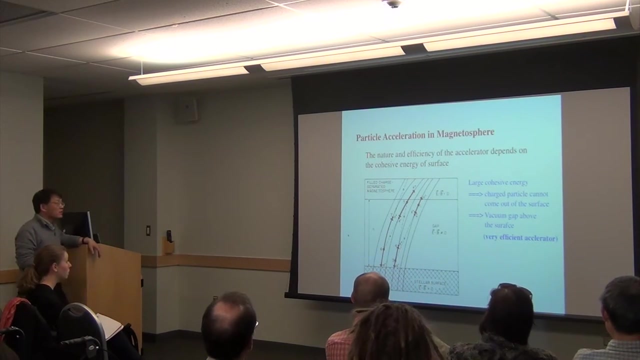 Right, This You know. how do you accelerate this? It turns out. how do you Where and how this particle accelerates in this manuscript depends on this property of the surface, At least under some conditions, right? The reason for this is that when you have a rapid rotation and magnetosphere, you can easily generate bottom electric field. 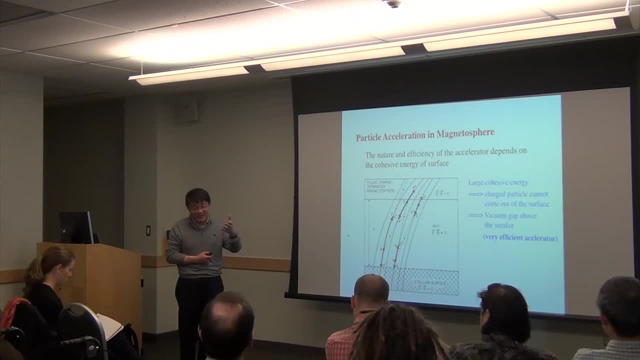 This is something you may You may get a hint about If you think about Faraday disk, if you study E and M electromagneticism, When you have a rotating rotation, you put a disk in the magnet field, You generate electromagnetic force. 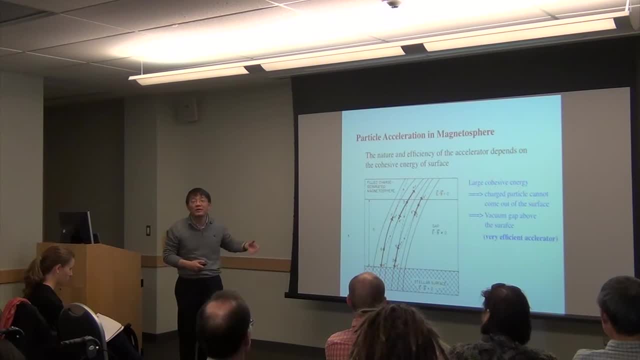 A lot of electric field, Like here. neutrons are the perfect combination of that Rapid rotation, strong magnet field and then you can generate a lot of electric field. So electric field- When you have a large electric field, you can pull charged particles out out of the surface. 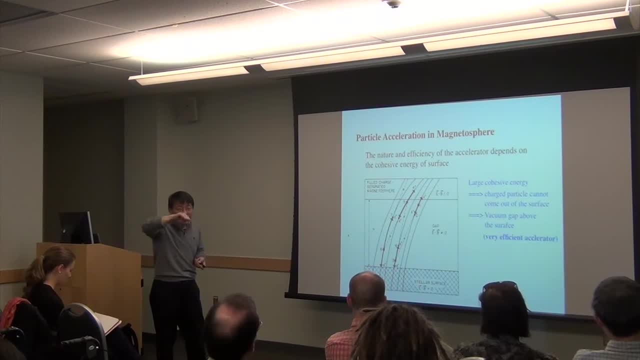 Right. So the ability to pull charged particles out of the surface Depends on how strong the solid is. Right? So if you have a very strong solid with high cohesive energy, then you can. Then it may be very difficult to pull charged particles out. 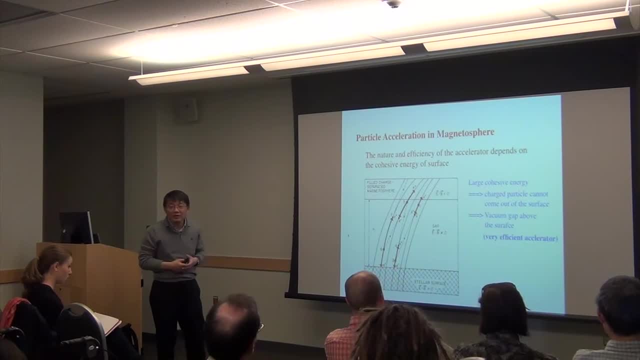 Then the electric field will be there, allowing you to accelerate particles and accelerate some other particles. On the other hand, if you have a weaker solid with weaker cohesive energy, then the particles can freely come out. Then you can short-circuit these things. 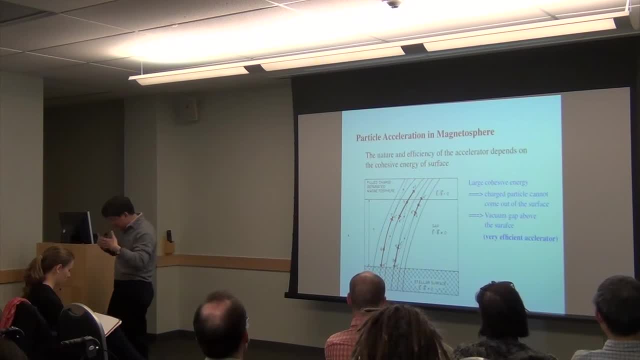 And you can. So again, I'm, I'm doing this. I'm talking about this in a very simple-minded way, But the general idea is the cohesive property of the solid will affect the accelerator that we know must be lying in the near vicinity of the neutron star. Okay, And so even this condensed matter, physics, can affect this problem. Okay, We have a weak field, We don't have a magnetic field, Right? This can only happen if we have a strong magnetic field. And another thing, Yeah. The vacuum itself becomes what we call birefringent, Namely it becomes a crystal, Even when you have a pure vacuum. but if you have a big field, the vacuum itself becomes birefringent. It behaves like crystal. The orbit is gradually shrinking on a time scale of several hundred million years. So we're not going to see it in our lifetime. but you know, next generation, Future generation, Anyway, it's going to decay, It's decaying. So the important part is the orbit decaying. Why is it decaying? Well, this is, of course, it's a prediction of Einstein's general theory of relativity. Einstein's theory of relativity predicted that when you have two bodies, two big bodies, orbiting each other. it's emitting gravitational radiation Right And it's gravitational radiation is at the expense of the orbital energy, So it's radiating energy there from the orbit is shrinking Right And this line prediction from general relativity agrees with the data point. You can see High precision. So of course, for so orbits, this thing eventually will shrink, And it's a strong prediction of Einstein's theory of general relativity. So of course, when eventually we have two neutrons that merge, something spectacular. can happen, Of course. here's a simulation from over a decade ago. People have done it in refining, but this is the first one. And two neutrons are coming close together, merge Methy-hydrodynamics process. Eventually, the combined neutron star collapsed to a black hole, leaving behind a little bit. of matter muonium-1.. This is a numerical simulation using full generative, using nuclear quotient state. Okay, And this merging process, when two neutrons are coming together, not so surprisingly, you can produce exotic phenomena, You can observe. And one of the phenomena you can observe is The And, of course, when they come together, they also emit very strong gravitational waves, In particular, of course, always radiating gravitational wave. When you have two bodies orbiting each other, you always radiating gravitational wave. But what's particularly interesting is that in the last three minutes of the binary's lifetime before they actually touch each other- the last three minutes, is that quite interesting? It emits gravitational radiation that can be detected directly And you probably pay attention to the news two months ago. And the last three minutes. it's emitting a gravitational wave with a frequency between ten to a thousand hertz- And that's a frequency band that can be directly detected by LIGO- And so emitting this quasi-initial wave of two of each other, emitting this spiral wave form. eventually, of course, two stars touch each other. it's a mess, And this is, of course, a gravitational wave, a general gravitational wave that can be detected, And, of course, a gravitational wave. it's always enough if you read enough videos. look at the video. If you read the last two months, you probably can see a lot of this kind of thing, because the big news for LIGO right Gravitational waves are the warpage of space-time, where you have these two bodies orbiting each other. and they perturb the space-time which propagate to us, our Earth, right. So what that manifests itself, gravitational wave manifests itself- is that when you have two test beds sitting there in free space, hiding there right, just sitting there forever. but if you're way passing by gravitational wave, passing by it perturbs the space-time such that the separation between the two test beds is going to oscillate. And that, of course, is how LIGO works, right, You have L-shaped interferometers, you have four test masses. when there are no waves passing by, the distance between this arm and this arm is equal to four kilometers, When waves passing by it perturbs the space-time such that the distance between this arm and this arm changes The function of time. so in the quasi in the periodic manner. so squeeze here, stretch there right, And this delta, the change of the relative length of these two arms- is equal to the dimension of number h times the length of the arm- four kilometers in the case of arm. So it's a very weak signal. we are talking about 20 minus 21,. so this is. you know, even with four kilometers, we are talking about length different in length, of 20 minus 21,. and 15th individual is much less, a thousand times smaller than the length of the photon. So how do you detect this? Because this is something very interesting in physics, in commando physics. we've talked about, Okay, and this LIGO thing, you know right, and, as you know, of course, two months ago they- well, you know, they announced the detection of quotation marks. two black holes, not neutral stars, two big black holes by the orbit of each other. they have been detected and they have it's. you know this is sensitive. they have not reached a dense LIGO yet, but they have been detected, okay. They have been detected and that was very exciting, of course. right So that one is two black holes, two big black holes. the way that you can detect it is that we have two big black holes, very big mass, 30 solar mass black holes. easy for the signal to join them. Neutral stars only have 1.4 solar mass, so you have to. you have to work harder to do the most sensitive thing. so so the hope is that in the next few years, with the, when the advanced LIGO reaches full sensitivity, you can detect neutral star binary up to 20, 200 megaparsecs and then you will be able to see neutral star merging or neutral star black hole merging. that will be very exciting, because when you have two black holes merging together, the only thing you see is quotation away. it's two black holes, nothing else. but when you have neutral star involved, you know neutral star with a black hole coming, the black hole, neutral star, will be ripped apart. the tidal is disrupted. and you. the violet is disrupted and neutral star or two neutral stars collide with each other. something dramatic can happen and see. you know you can. you can heat up the matter. you know you can emit gamma ray radiation. electromagnetic radiation and actually do some real astronomy with it, right. So so the hope is that this stay tuned. I think this may should happen in the next five years, hopefully detecting neutral star merging with a neutral star with a non-neutral star. and or neutral star- black hole merging. And finally, of course, going back to my theme that using neutral star to probe extreme physics, you can probe, for example, property of neutral star using the disruption- tidal disruption- When neutral star get disrupted by black hole. the property of nuclear matter is embedded in the quotation wave signal. By looking at those properties, those signals give you another way to probe neutral nuclear matter. Okay And okay, that's my final slide. so I have- I hope I have- sort of give you some flavor of the, the kind of exotic thing we're studying. a lot of fun, I think. neutral star, neutral star, white hole, black hole, a lot of different things that are going on right To understand these things, these objects. these different manifestations, of these different kinds of things we have to. you know we study all kinds of things, Right, You can, if neutral. in particular, it has become a very good laboratory to study physics under extreme conditions, measuring neutral star mass radius. you can get neutral star equation state and you can study- I did not talk about some of these nuclear- how they hold neutral star cool, how they cool down over time and that they have important applications. So thank you, That's it. 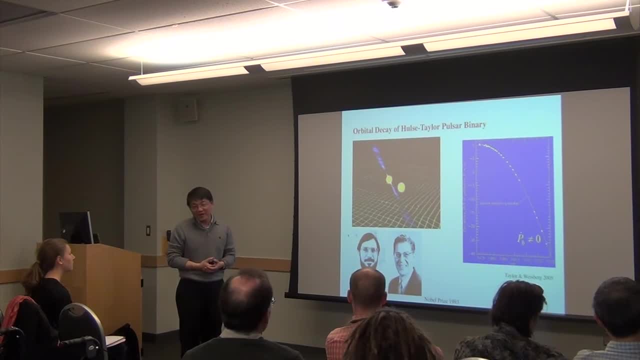 So thank you, Dom, for this very engaging talk And if you have any questions, So what causes the strong magnetic field in the neutral star? to start with, Great question. I was asking that. Okay, It's well, there are several ways. I think the simplest way is just: you know, the sun, Most of the stars, Most of the stars have a magnetic field. Okay, Earth has a magnetic field. So, since I don't know anything about astronomy, why do the stars? you know what causes the magnetic field. 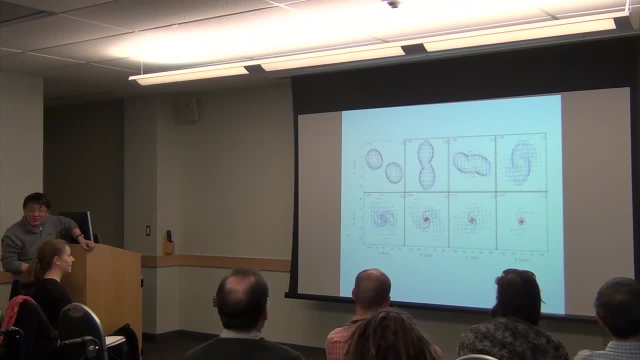 So strong. Why so strong? That's right, Okay, So the simplest way, simplest, one of the standard textbook pictures is that all stars have a magnetic field, to some degree- Weak. one right, Earth has a magnetic field. The sun has a magnetic field. 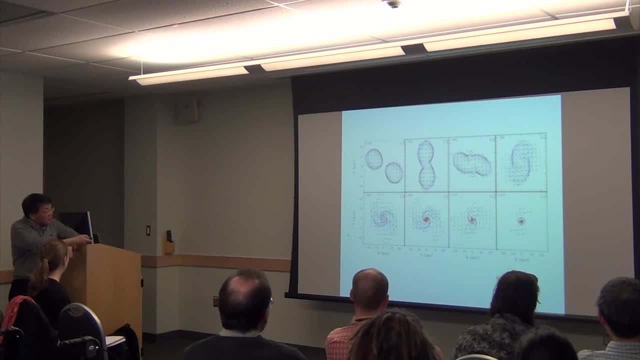 Right, The sun, the surface has a magnetic field, And the massive star, which is the progenitor of neutral star, they have a magnetic field. Okay And okay. and this object normal stars. they are very puffy. 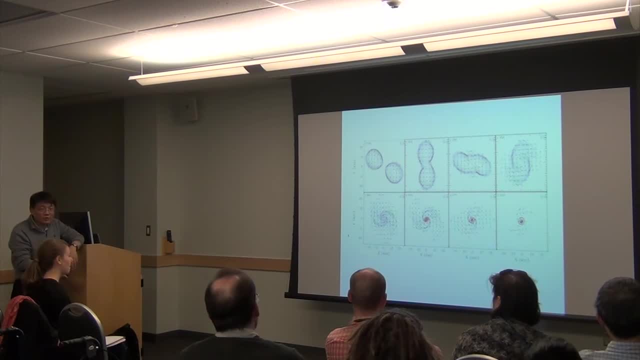 They are very big. But now, if you imagine collapse this thing, Shrink this, collapse this, this, this- to form neutrons out of an ordinary star. you have to shrink the thing inside, Compress it. They have to collapse. 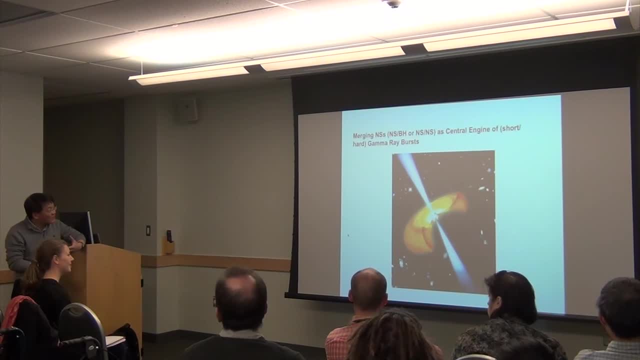 Right, There are many other manual compressions we're talking about. Okay, So now, if you have a good conductor, if you have a good conductor, you better have a good conductor. When the matter collapse, it actually drags the magnetic field line with it. 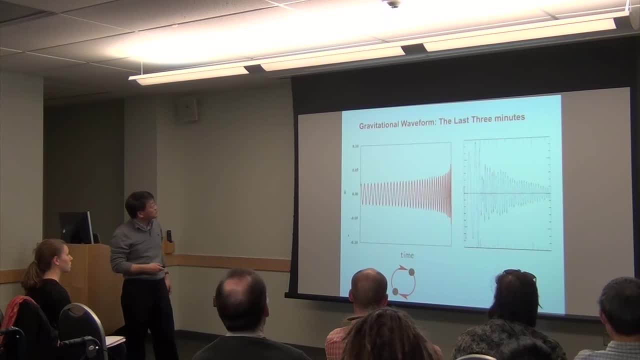 Conserving the flux. It's called flux conservation. This happens when you have a very good conductor. When the matter force, the field line gets dragged together with it. So flux is conserved, So B times the area is conserved, So B times the size squared is conserved. So, given the initial field weak in the normal star stage, r is large. if you reduce r, the b were increased by the ratio of radius squared. so that's one way to generate very strong magnetic field. for in that sense it may not be so surprising that this most compressed object had very strong. 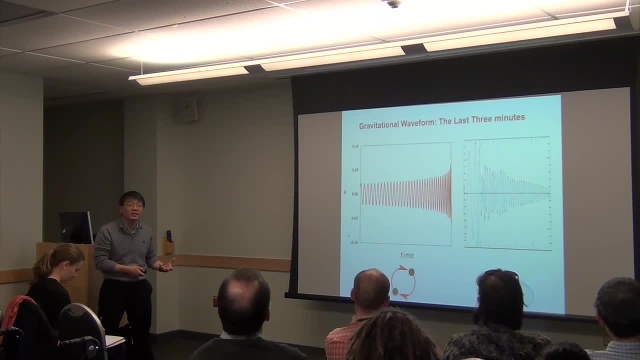 so in the case of, am i correct that people think that i don't know some iron in the earth's core or something like that? oh, okay, okay, so to have it, to have it, i don't have to make that field, you need a current electric current. okay, so you have, you need an electric current. so, in fact, neutrons. 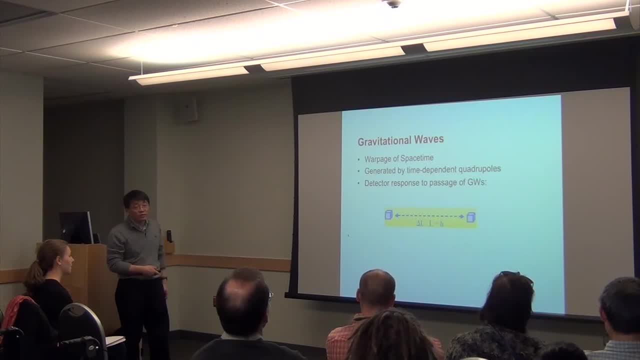 start a certain electric current. so what you need is to have electron photons who have slightly different drift, at different speeds. they're all moving but they have slightly different speeds. so you have, you need a current. so the current electric current that responsible for the b field could lie in the center of the neutron star. basically, you have electron proton. 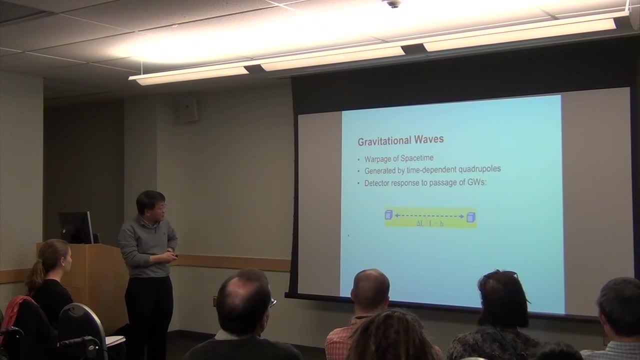 all you need is a move right to each other, right, right. if you have a plasma, you have an ionized everything to ionize, you have electron protons. by the way, another thing i did not say: even though we call, even though we call this neutron star, it's actually not pure neutron star. 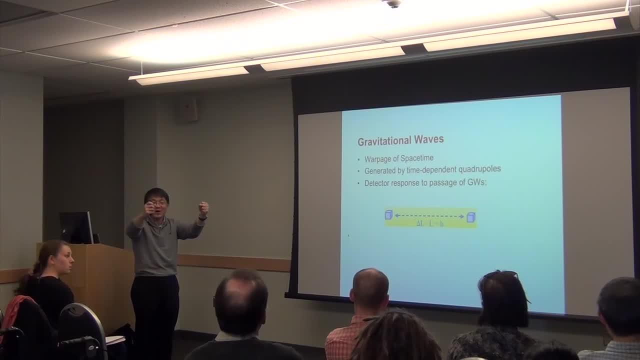 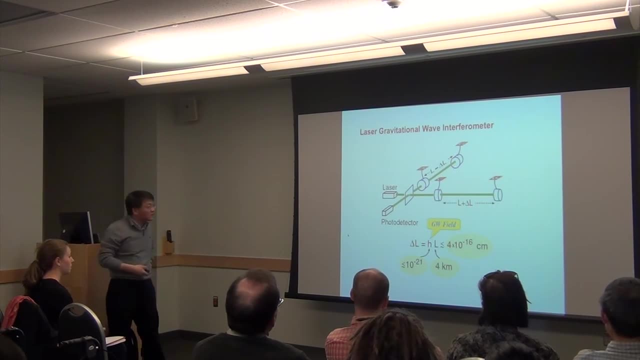 if you actually have electrons and protons, a small fraction, mostly neutron, but you still have electron proton. so when electron proton has slightly different bulk velocity, drift velocity, you have an electric current. so it is this current electric current that responsible for the b field. now, as to where the current lies, in the center or in the cross or in the outer region- then 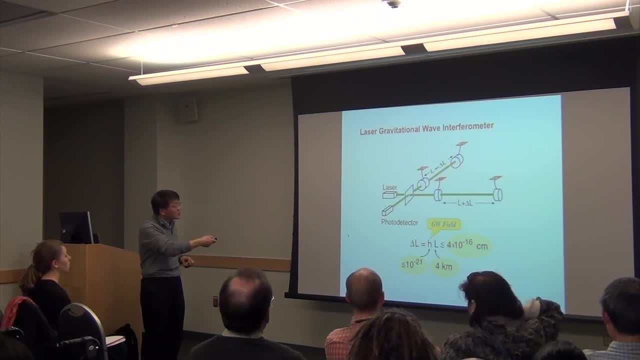 we don't do anything. okay, so it's automatically electric current, right? so what i said earlier, what response? what's generating those currents? maybe due to this flux? is well, electric current is like orbital currents, like in atoms, or could be. no, not necessarily no such, it's just a bulk motion. 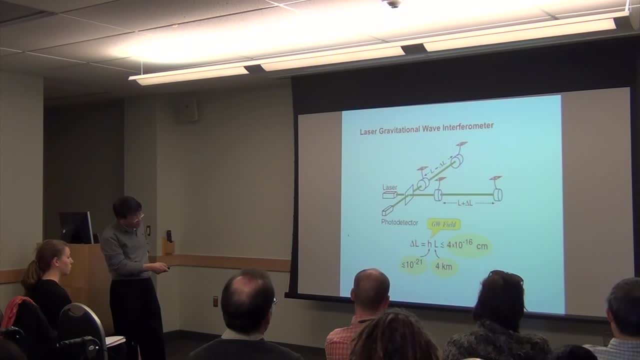 by the way, when you have such high density- the concept, when you're in the central region, it's all squeezed, everything is ionized. i talked about atom made earlier on. it's near the surface. when you go to the bulk region of the star, everything is squeezed. 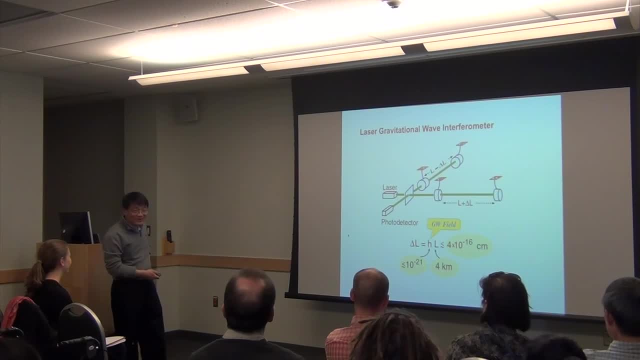 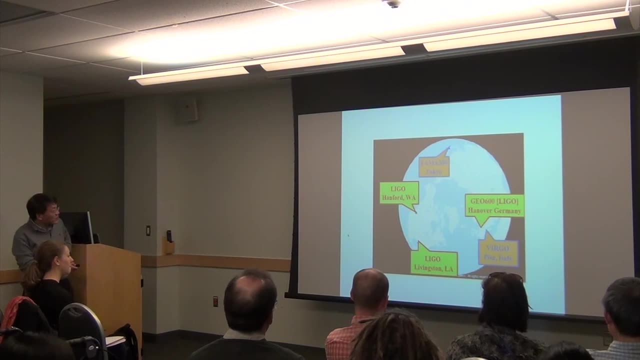 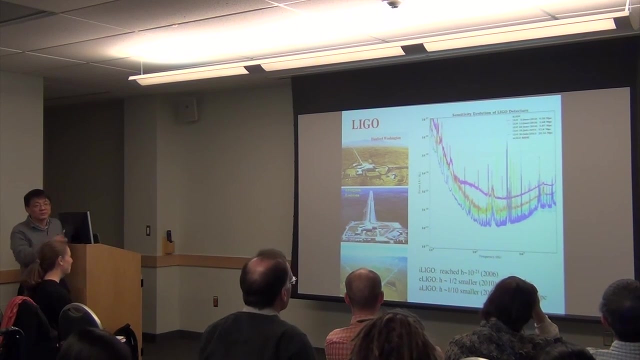 everything is ionized. so the motion is not the. it's not the, it's really the motion, bulk motion of electrons and protons. they don't move the bulk, large-scale motion. this is what's happening to the earth, also the earth's core. you know the electron, you know from the moiting core there's. 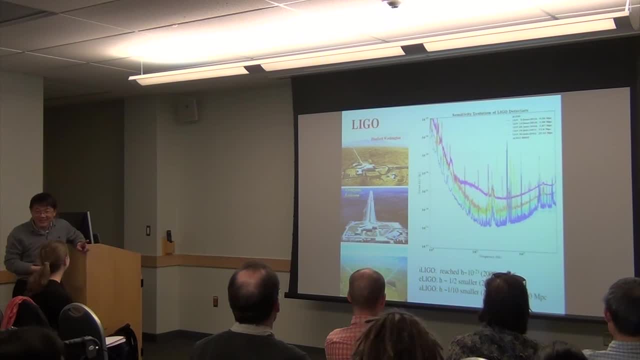 very electric current. ultimately, the current is due to motion, relative motion to electron ions. any further questions? what percentage of the neutron core is actually protons? one, two percent, one to two percent? yes, so this is all that. we call that neutron stuff. you cannot have pure neutron stuff. this is actually very small percentage. that's why you call it neutron.